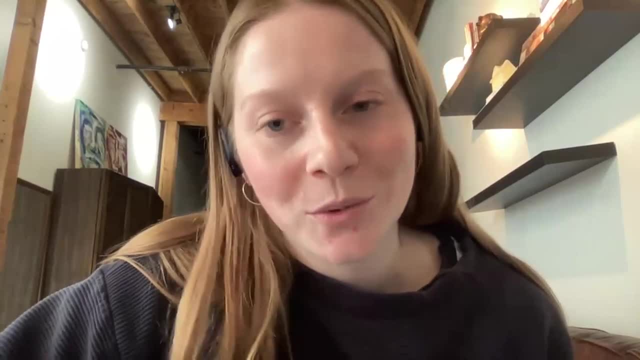 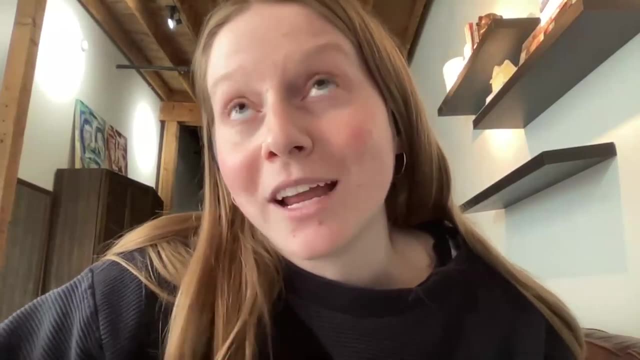 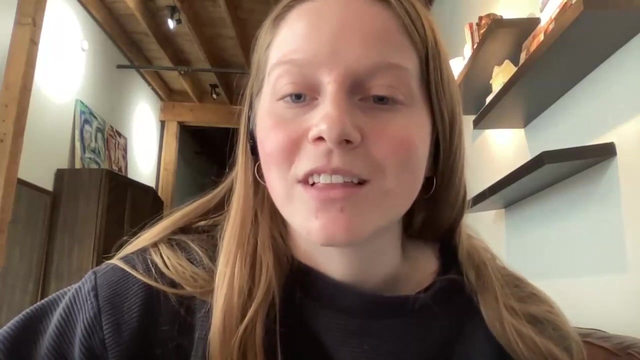 Tori Thorpe, who is our field biologist, currently pursuing her master's at Utah State, and then we are going to hear from Dr Fidel Atuo, our HWI board member and also assistant professor at the Southeast Missouri State University. We are going to save the last five to ten minutes for question. 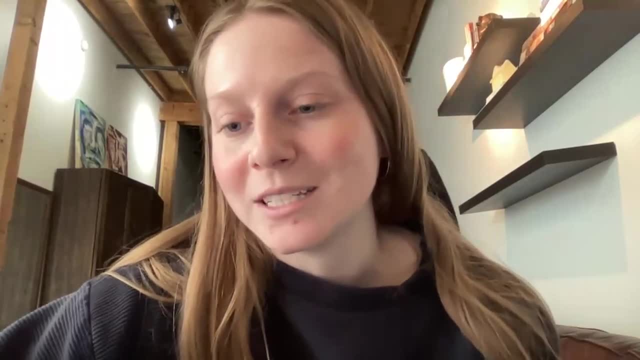 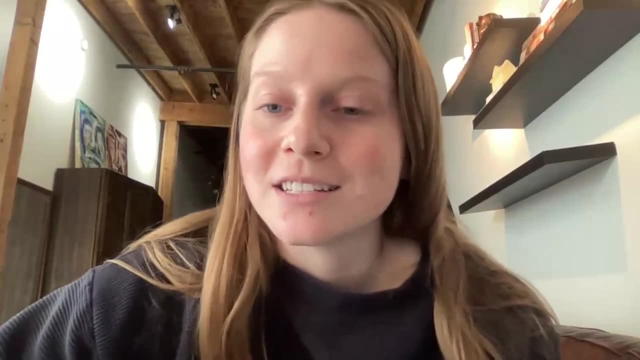 and answer, so if you have any questions throughout the event, please put them in the chat. I want to say that we are able to offer this programming for free thanks to ZAP funding for those of you who are local to Salt Lake County, and with additional support from donors like you. 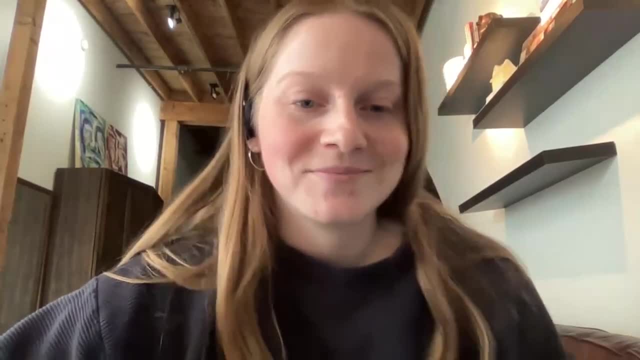 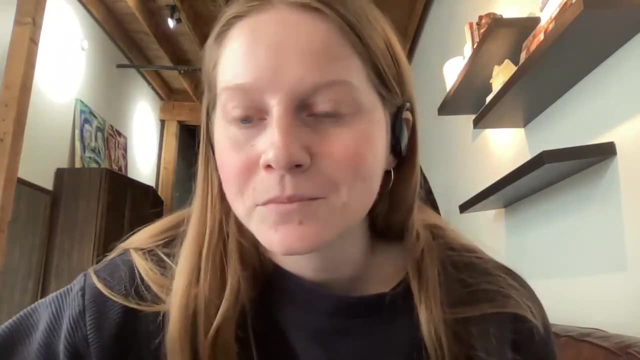 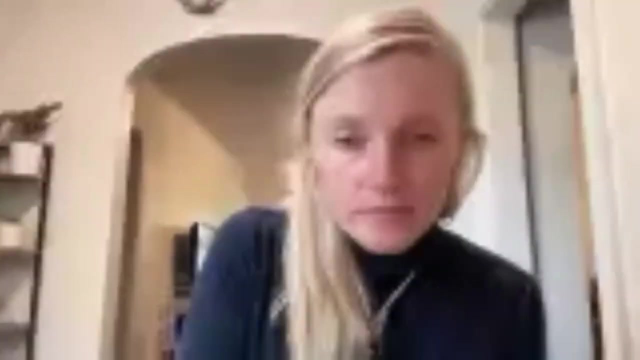 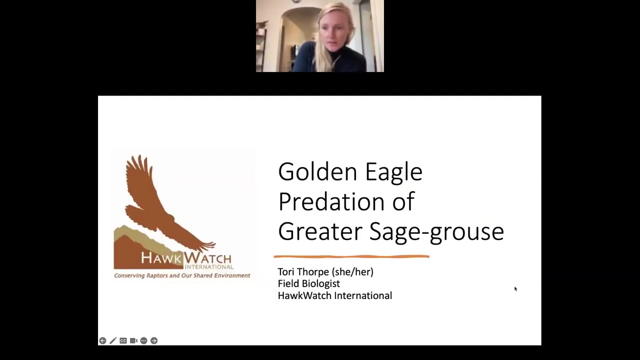 So with that, I'm going to turn things over to Tori. Hi, everybody, I'm going to get my screen shared here with you, All right. So, as Sammy mentioned, I'm Tori Thorpe. I'm a field biologist at Hawk. 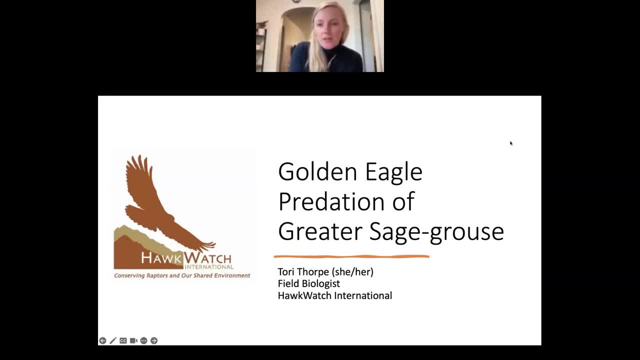 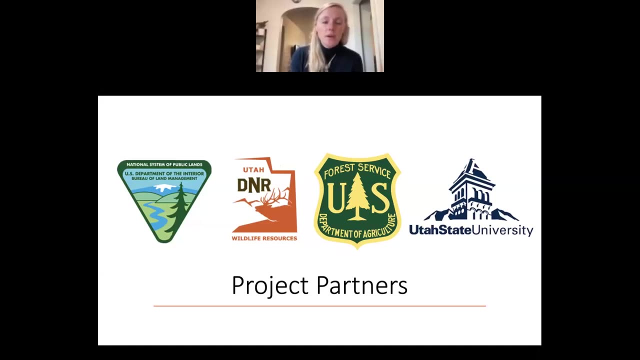 Watch International and a grad student at Utah State University, and today I'm going to be talking to you about golden eagle predation of Greater Sage Grouse. My partners on this project are the vernal offices of the Bureau of Land Management, the Utah Division of Wildlife Resources, the US Forest Service and Utah State University. So, first off, if you wanna do a short video, kind of listening to this content right now is what you're going to do is send me a video request or a SSL email. So if you wanna add a question or 1988, or a review, it will clear your mind before we record this. You're free to do so. for now, I'd sorta move on. So here are the things we have in our document. just run and screenshot this question for good reason, But if you'd like to comment on it, 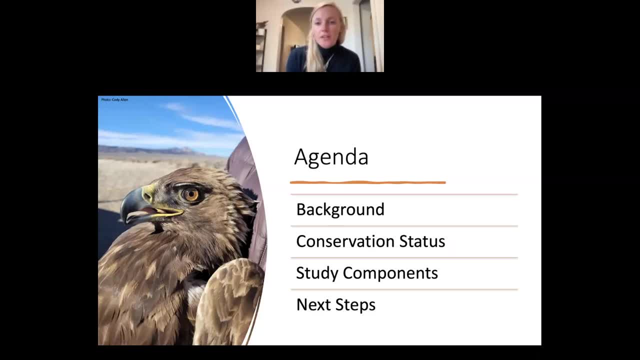 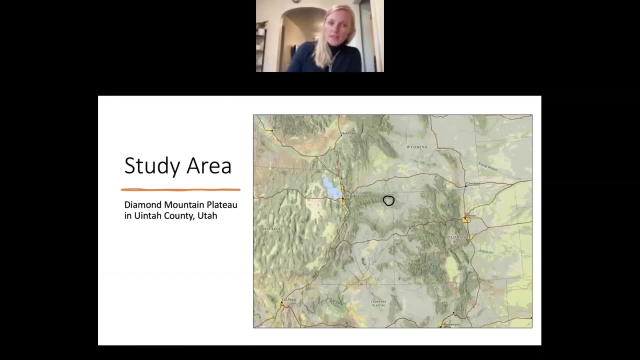 first I'm going to give you some background information. We're going to talk about the conservation status of golden eagles and sage grouse and my study components for this project, and then conclude with the next steps of my project. So my study area is the Diamond Mountain Plateau, located in Uinta County, Utah. For those of you, 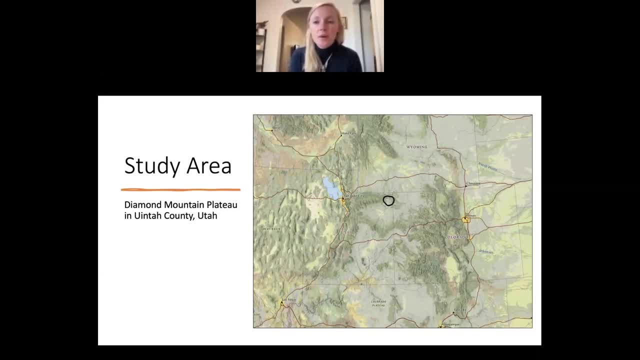 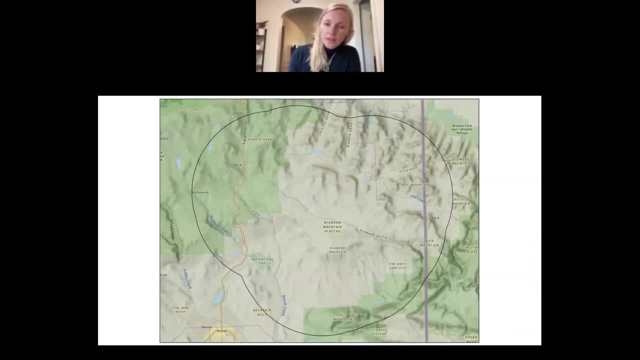 not familiar with Utah geography. it's in the northeastern part of the state, close to the Colorado and Wyoming borders. Here is a zoomed in map and you can see Diamond Mountain Plateau in the center there And this area has federal, state and private land And this black line. 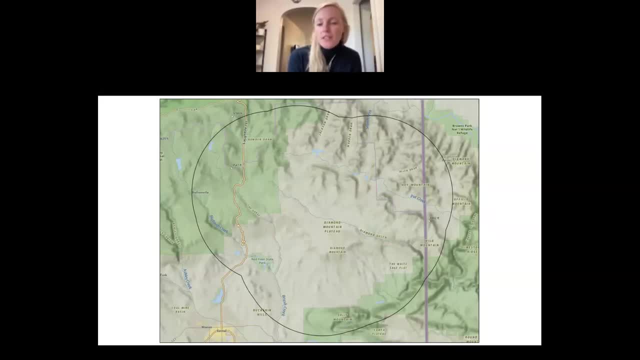 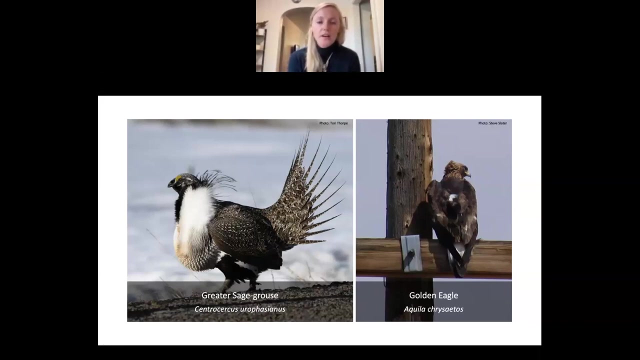 represents a 10-mile radius of the Lex On Diamond Mountain Plateau, and in that area I'm searching for golden eagle nests, because there's not a lot of great nesting habitat on the plateau itself. So the two species of my project that I'm focused on are the greater sage grouse and the golden eagle. 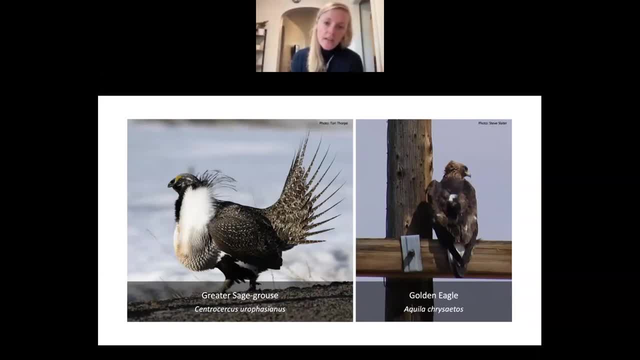 And this is a picture of a male sage grouse here on the left and he is strutting along the side of the road. And this is a picture of a male sage grouse here on the right and he is strutting along the side of the road near one of the leks. 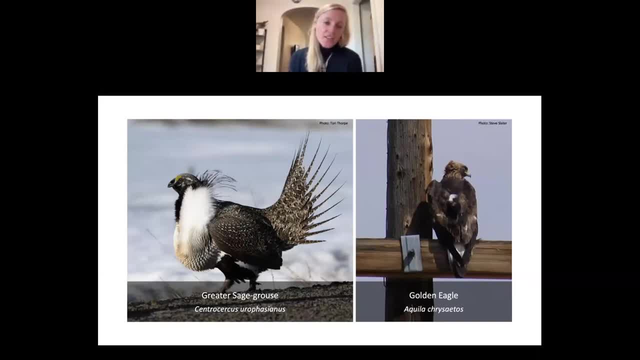 Greater sage grouse are the largest North American grouse species and one of only two sage grouse species in the world. The other is the Gunnison sage grouse. The golden eagle is one of two species of eagles we have in North America, the other being the bald eagle. 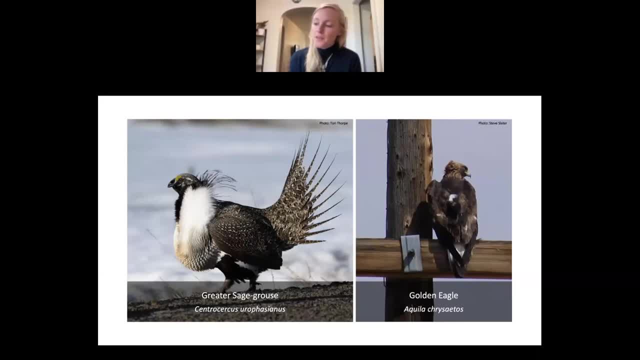 And they're found throughout the western US and Canada and inhabit a variety of different biomes In the sagebrush ecosystem. they can be found as year-round residents. Golden eagles are one of the natural predators of greater sage grouse. 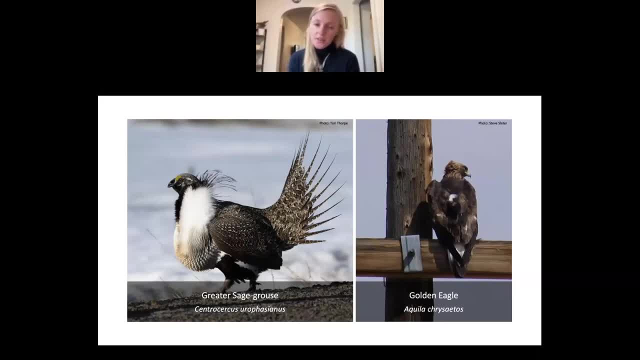 And other predators of adults include coyotes, great horned owls, red foxes, northern goshawks, bobcats, red-tailed hawks, feruginous hawks, Swainson's hawks and Cooper's hawks. And although many species will eat sage grouse, no one species specializes on predating them. Although golden eagles do predate sage grouse, lagomorphs generally constitute the largest proportion of prey in golden eagle diets And, if you're not familiar, lagomorphs include rabbits, hares and pikas. 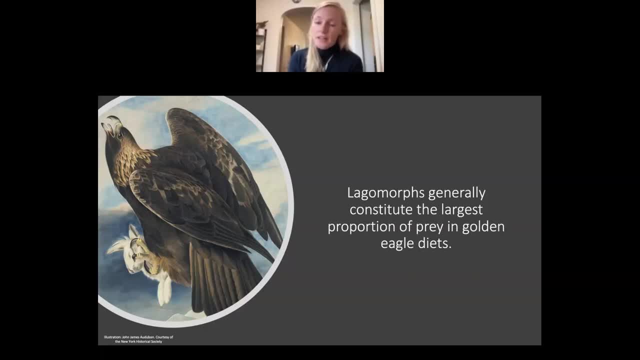 And the abundance of lagomorph is cited as one of the critical factors affecting golden eagle reproductive success. Although predation of sage grouse is not a common practice, it is likely to play a significant role in the decline of sage grouse. Few observational studies have focused specifically on golden eagle predation of sage grouse. 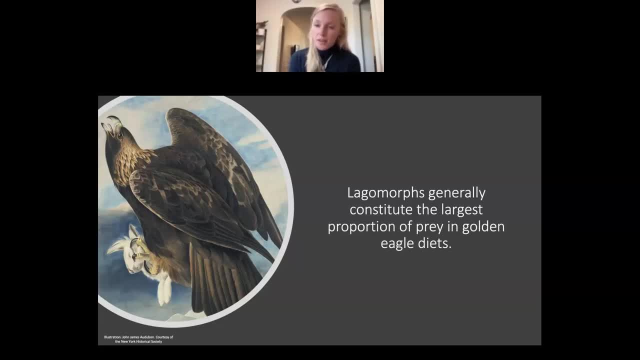 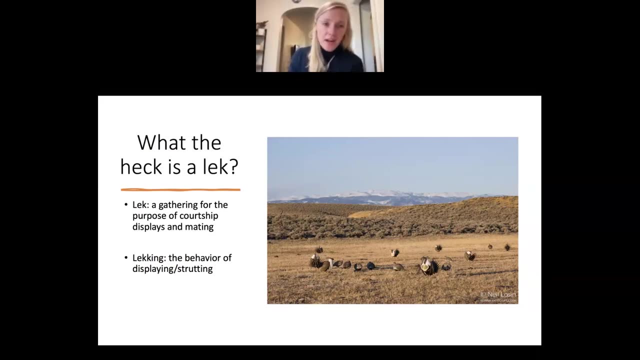 or sought to quantify sage grouse response to golden eagles during the lek period. So at this point, you've heard me say lek a bunch of times And if you're not familiar, a lek is a gathering for the purpose of courtship displays. 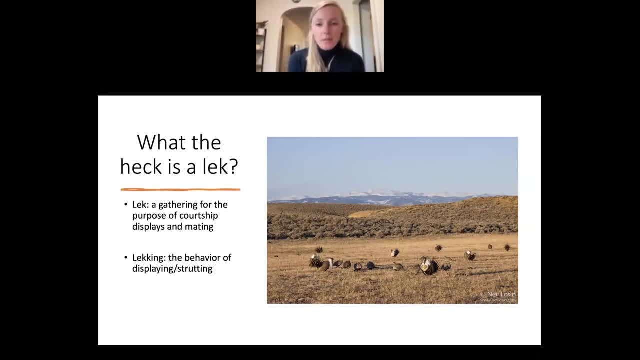 and mating, And lekking is the behavior of displaying and shredding. Counting. annual male attendance has served as the primary means for monitoring sage grouse populations for more than 80 years, And generally these lek areas are flat, open areas on the prairie, as you can see here in this photo. 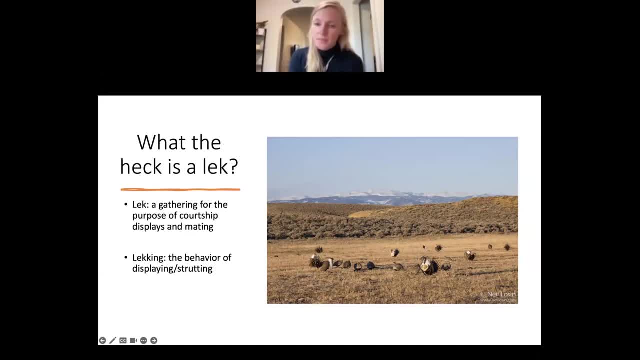 And the lek period occurs from March through the middle of May, And the birds will start gathering at first light and they'll continue their displays a few hours after sunrise. This is when males are most vulnerable to predation, And that's because they're coming out of the cover of the sagebrush and displaying. 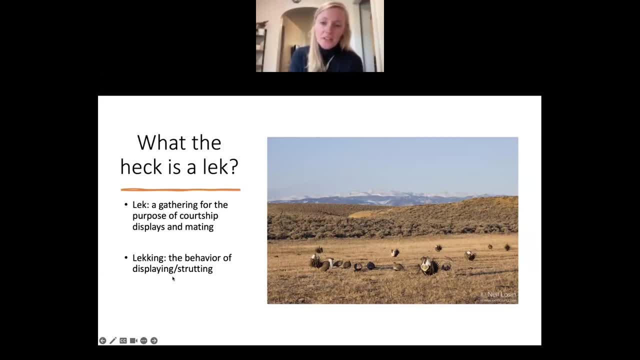 And that's also why they're easy for land managers to count them. Quantifying how sage grouse react to various predators at the lek and the duration of those responses will provide more information on the relationships between sage grouse and their predators during the lek period. 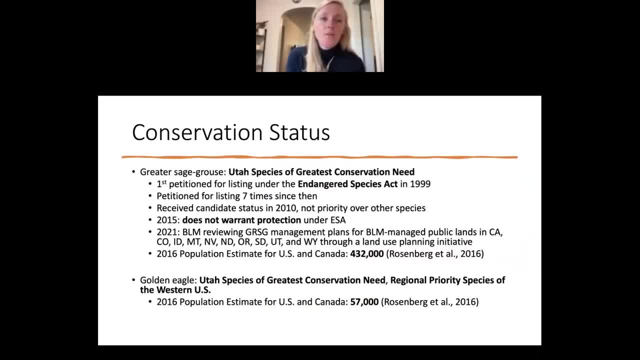 That's about it for this video. Now I want to talk a little bit about the conservation status of both sage grouse and golden eagles. Greater sagegrouse are considered a Utah species of greatest conservation need And the federal status is a little bit more complex, as you may have heard in the keynote. 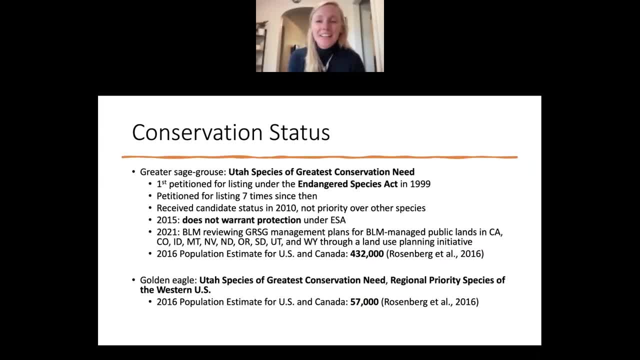 And that's because the conservation status on those species is relatively limited, heard in the news the last decade or so. They were first petitioned for listing under the Endangered Species Act in 1999 and have since been petitioned an additional seven times In 2010,. they received 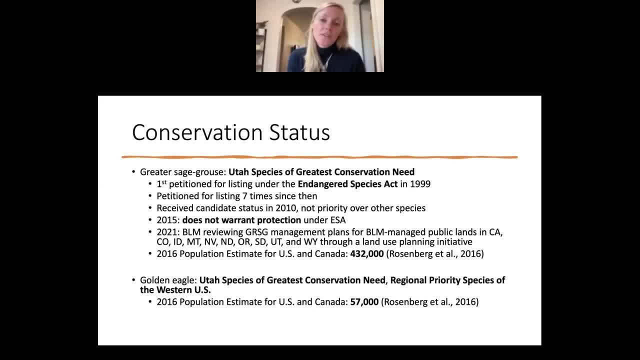 candidate species status but were ruled as not a priority over other candidate species. In 2015,, the US Fish and Wildlife Service announced that greater sage-grouse do not warrant protection under the Endangered Species Act. The most recent update is in 2021, the BLM announced. 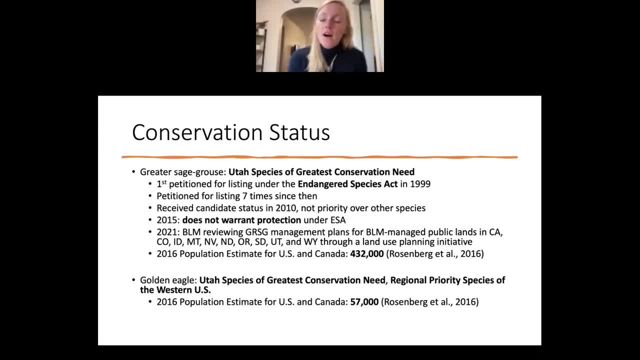 that they're reviewing greater sage-grouse management plans on BLM-managed public lands. This is really important because the BLM manages the largest proportion of sagebrush habitat and the BLM-managed public lands are the largest proportion of sagebrush habitat. 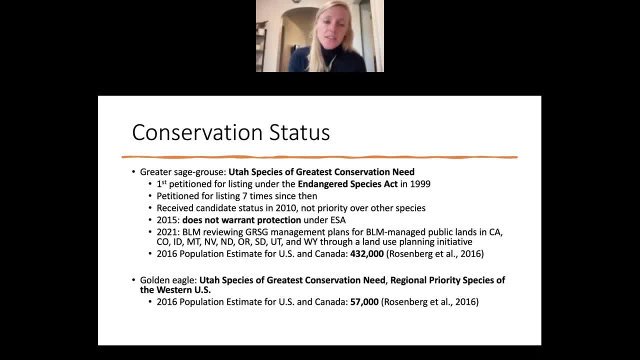 In the United States. a 2016 population estimate for US and Canada is around 432,000 individuals. The golden eagle is also considered a Utah species of greatest conservation need, as well as a regional priority species of the western US. A population estimate from the same source estimates there to be about 57,000 individuals in the US and Canada And, as you can see, there are a lot fewer golden eagles than sage-grouse. This is a pre-European. this map shows both the pre-European sage-grouse distribution. 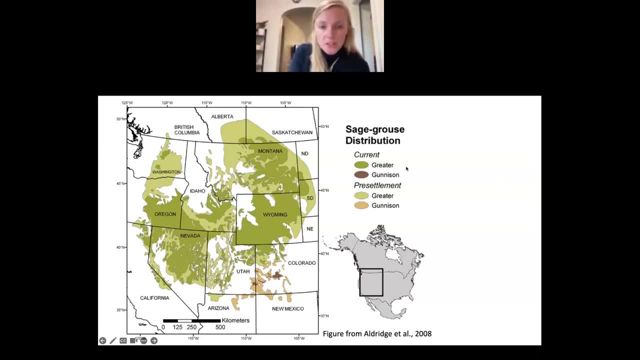 compared to the current sage-grouse distribution. So you can see the light green represents pre-settlement And the dark green is the current estimates. So you can see that currently they're occupying a lot less area than they were prior to European settlement. 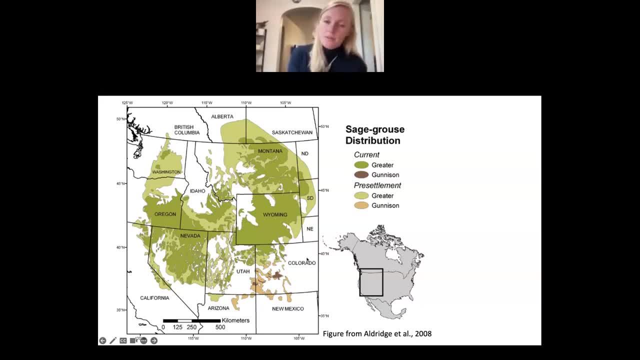 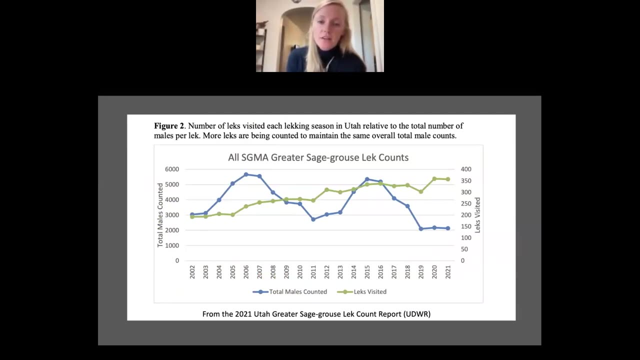 And they've been extirpated on the periphery of their range in states including Arizona, Nebraska and parts of British Columbia. As I mentioned before, counting male sage-grouse at leks is one of the primary means for tracking populations long-term. 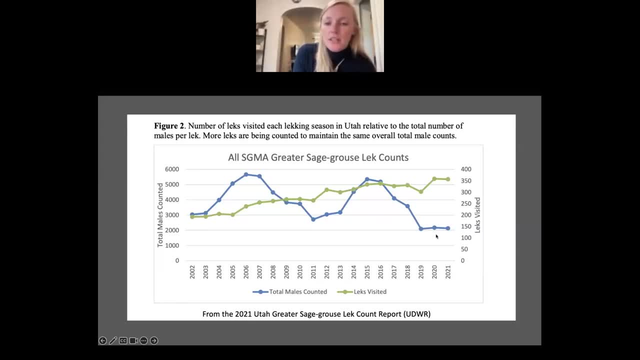 And this is a figure from the 2021 Utah Greater Sage-grouse Lek Count Report And you can see here, over the last 20 years we've had ups and downs in the population estimates, But specifically the last three years we've seen a lot fewer males. 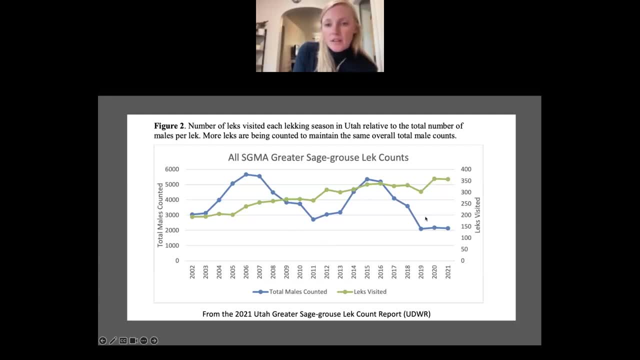 And that is because the number of females, especially in the 250s and the 60s, have been counted at the leks, And this is really interesting compared to the number of leks visited each year. So, despite more and more leks being visited by wildlife managers, each year, we're seeing fewer males overall. 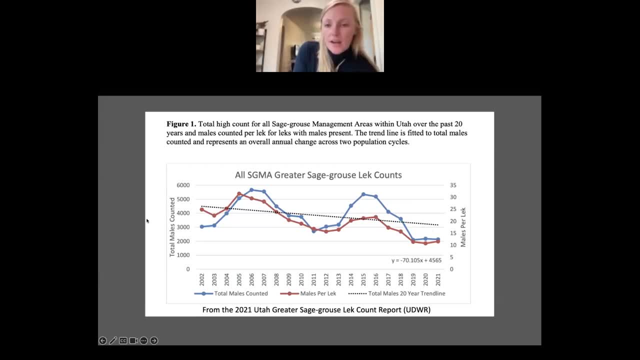 This is another figure from the same report And this one gives us a nice trend line of the last 20 years showing a general decline in grade 2.. And this one gives us a nice trend line of the last 20 years showing a general decline in grade 2.. 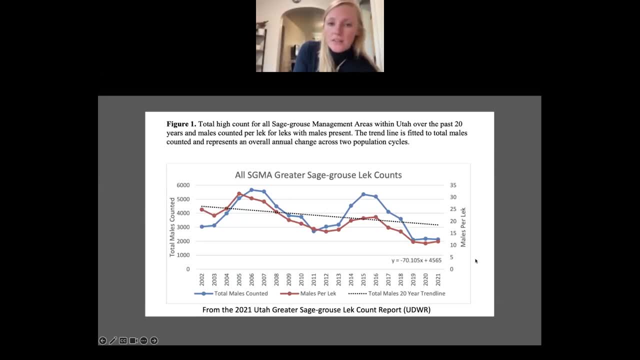 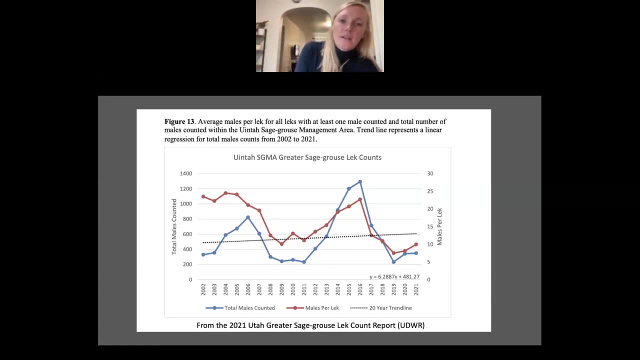 decline in greater sage-grouse lek counts throughout the state of Utah. This is the same figure except for the Uinta County sage-grouse management areas, which is the county where my study is located. And one thing that's really interesting is: you see the same. 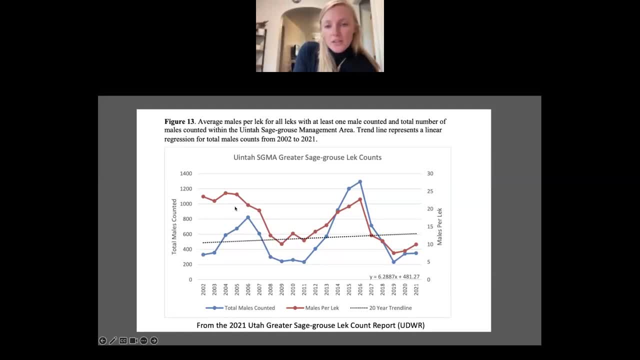 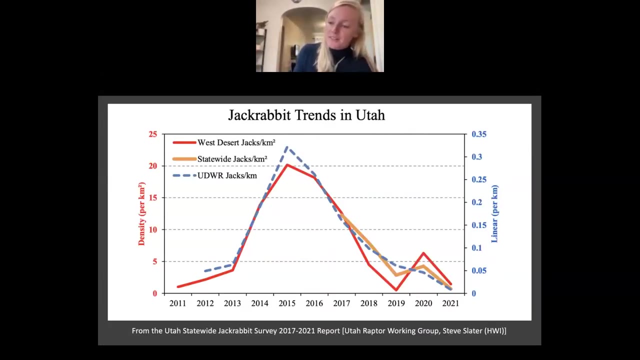 ups and downs in the lek count trends, but there's actually a slight increase over time in male attendance at the leks. As I mentioned before, jackrabbits and other rabbits are the primary prey source of golden eagles, And rabbits also have a similar cycling pattern to sage-grouse. 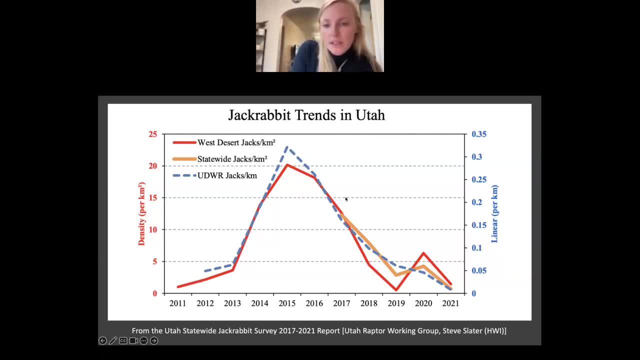 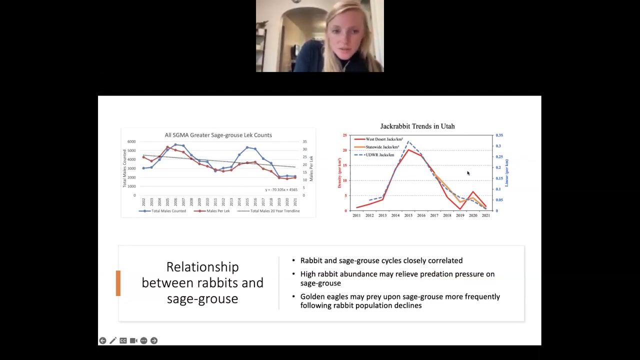 and you can see that in 2015 and 2016, they experienced a similar height of population and the last few years we've been seeing an overall decrease in the rabbit counts throughout the state of Utah. Here I have those two figures side by side, where you can see that in 2015-2016,. 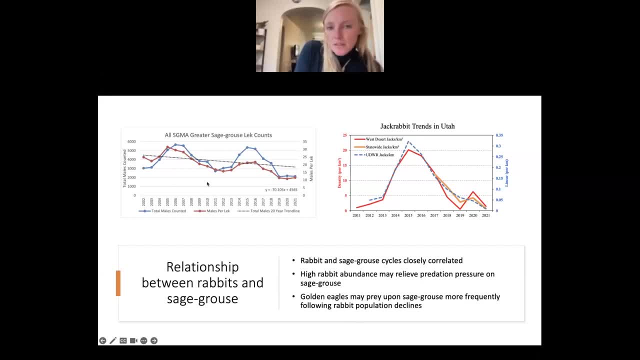 both rabbits and sage-grouse experienced peaks and then, the last few years, that overall decline. Several studies have found that rabbit and sage-grouse cycles are closely correlated, and that's really important, because a high rabbit abundance may be a factor in sage-grouse. Alternatively, golden eagles may prey upon sage-grouse more frequently. 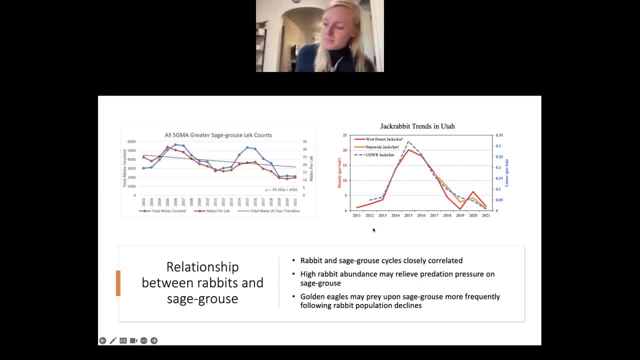 following rabbit population declines Due to the complexity of ecological relationships between cyclical species that share a predator. examining the rabbit populations on Diamond Mountain may yield some interesting information about the local relationship between rabbits and sage-grouse. Now maybe you're thinking: why are sage-grouse declining? 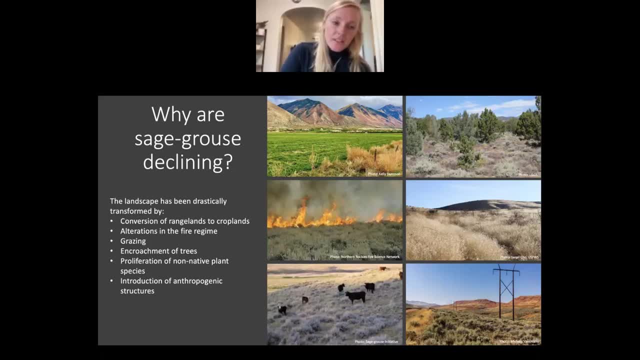 And, as I've previously mentioned, it is unlikely that golden eagles are a significant contributor to the decline in sage-grouse, and it's really important to think about all the changes in the landscape that the sagebrush ecosystem has seen since the arrival of European settlers. 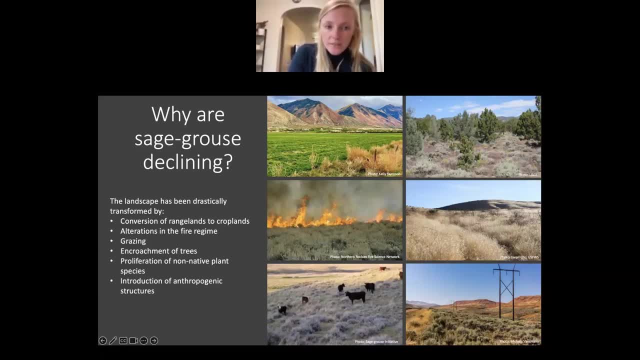 These changes include conversion of rangeland to croplands, alterations in the fire regime, where we're seeing some areas of the landscape change, and some changes in the climate, such as the climate change areas burn much more frequently and other areas not being burned at all, grazing encroachment. 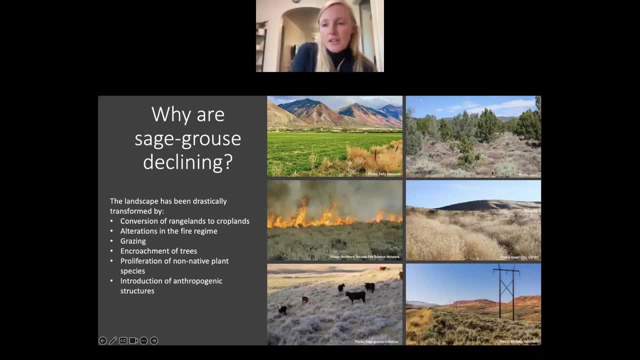 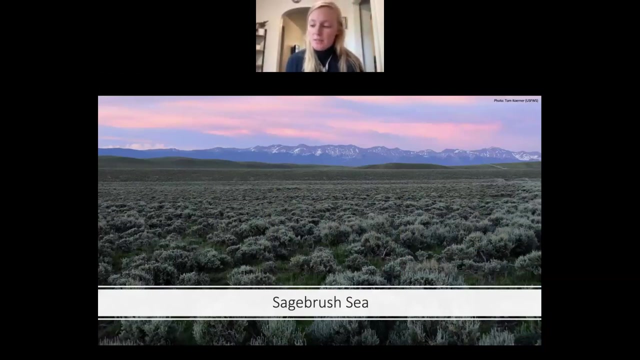 of trees, specifically pinyon, pine and juniper. proliferation of non-native plant species, especially cheatgrass, which you can see in the middle right photo, and the introduction of anthropogenic structures. So, historically, the sagebrush landscape was characterized by vast open expanses of 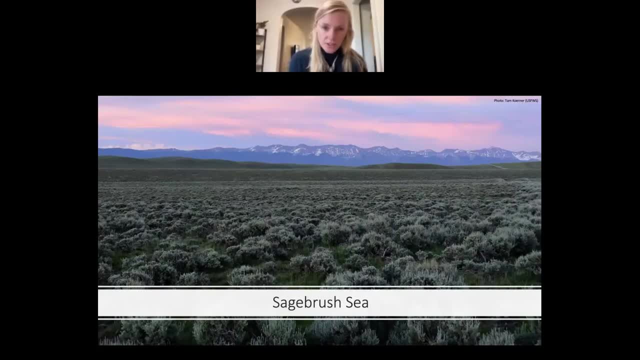 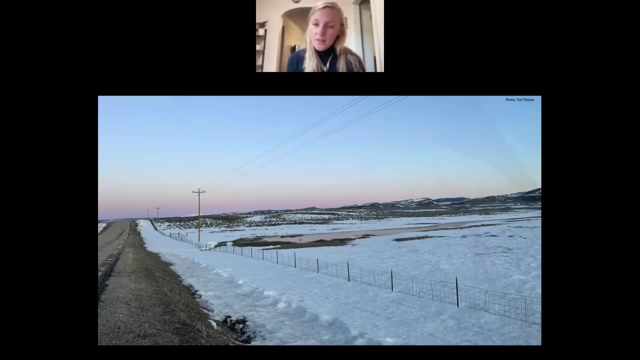 sagebrush with very few trees or tall structures. Today, the introduction of anthropogenic structures such as telephone poles, fences, power lines, transmission towers provide structures for raptors. These structures can be used as perches and nesting structures. Previous research has investigated the impact of tall structures and the increased risk. 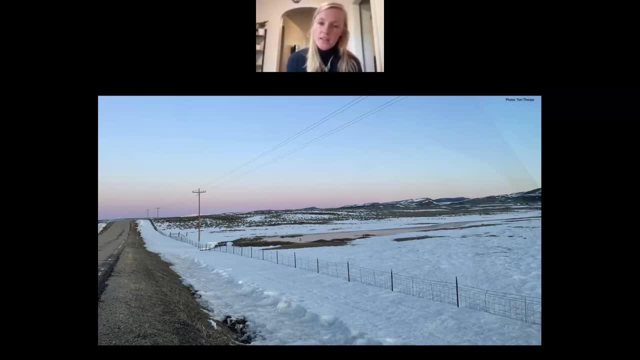 of predation of sage-grouse, but they often do not assess the proportion of sage-grouse in predator diets relative to other prey species. There are still knowledge gaps on the influence of tall structures on the direct raptor, predation of sage-grouse and other possible negative effects on sage-grouse. 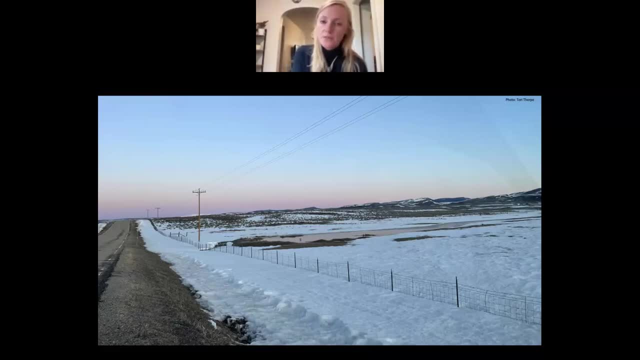 This photo is from one of the leks on Diamond Mountain in my study area. You can actually see on the ice there's a sage-grouse and this lek is split by a road and power lines and two different fence lines, one running parallel to the road and one running 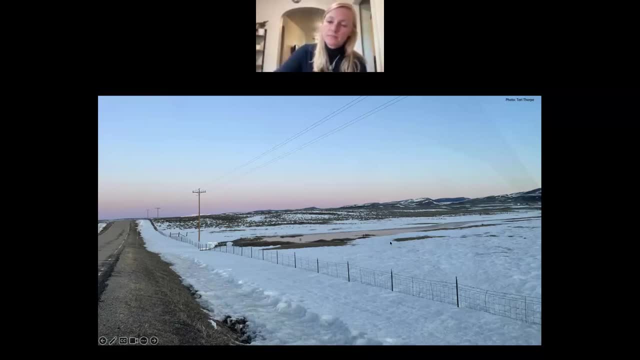 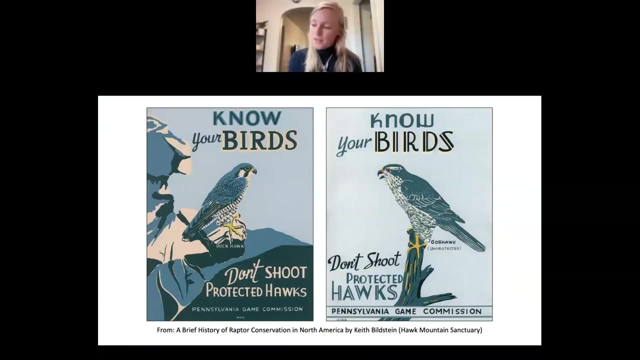 perpendicular. Although understanding raptor predation is really important to understand their effects on sage-grouse, it's really important for us to keep things in perspective. Predators, including raptors, have often been viewed negatively because of their ability to take livestock and compete with hunters for wild game. 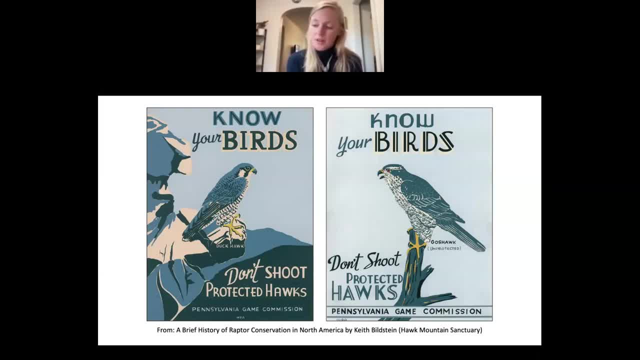 In Europe, raptors have been persecuted for centuries because they are viewed as competition to game bird hunting. I found these posters- This is from the Pennsylvania Game Commission- to help hunters separate good hawks, like the peregrine falcon on the left, from bad hawks, like the goshawk on the right. And until 1951, the Pennsylvania Game Commission even had a bounty for $5 on goshawks. Today, golden eagles in the US are protected by the Migratory Bird Treaty Act of 1918. And the Bald and Golden Eagle Protection Act of 1942. 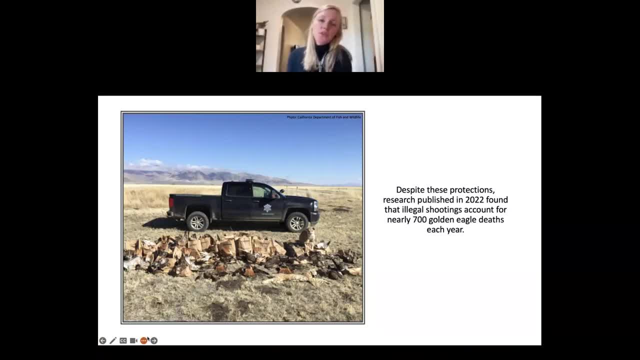 But despite these protections, research published in 2022 found that illegal shootings account for nearly 700 golden eagle deaths each year And, due to their protection status and conservation status, it is an unreasonable management solution to consider removing raptors for the benefits of sage-grouse. 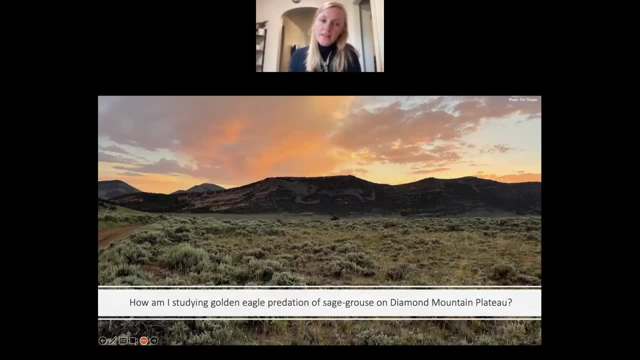 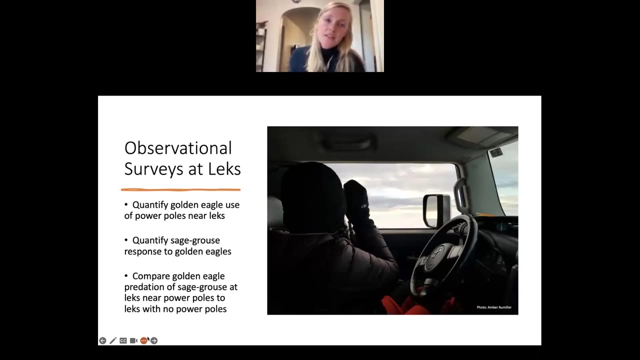 Now that I've given you some background info, I want to talk about how I'm studying golden eagle predation of sage-grouse on Diamond Mountain Plateau. One of the main components of my project is conducting observational surveys at leks, And this includes counting male lek attendants as well as female lek attendants and also. 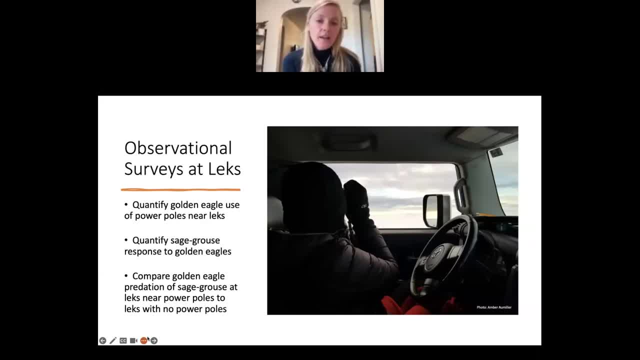 identifying all predators. We're also looking at predators close to the lek, how far away they are from the lek and how much time they're spending near the lek. And we're also looking at predator behavior: whether they're flying through, perching on. 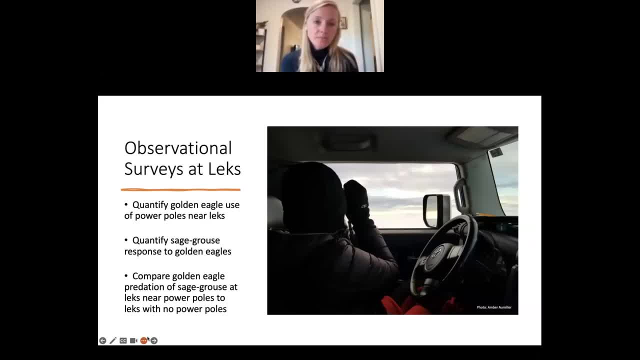 power poles or on natural features, And I'm hoping to use this data to quantify golden eagle use of power poles, specifically during the lek season, and quantify sage-grouse response to the presence of golden eagles, Thank you. Then I plan to compare golden eagle predation of sage-grouse at leks near power poles to 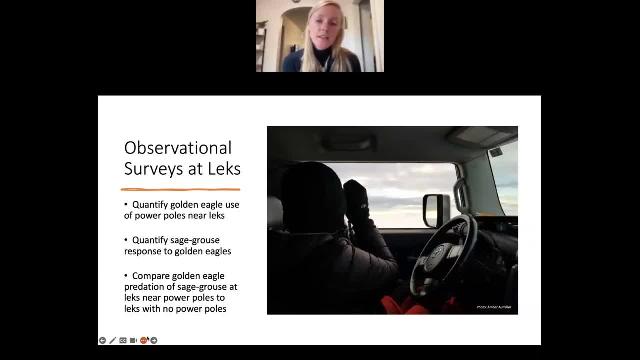 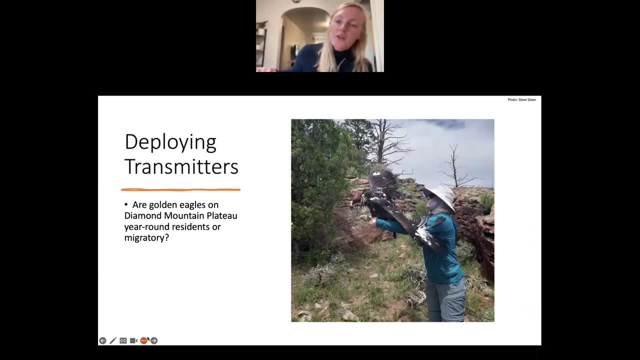 leks with no power poles, to help understand the impact of anthropogenic structures. I'm also deploying transmitters on golden eagles in the study area, And this is to help answer the question of whether or not the golden eagles on Diamond Mountain Plateau are year-round residents or migratory eagles. 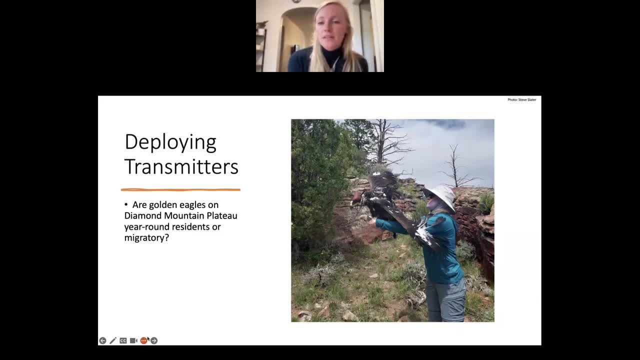 And I'm hoping to use this data to quantify golden eagle predation of sage-grouse at leks. The lek period coincides with the timing of spring raptor migration, So I'm interested in whether or not eagles spending time near the leks are passing through. 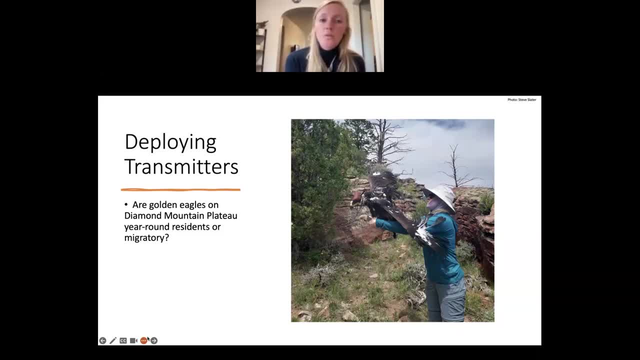 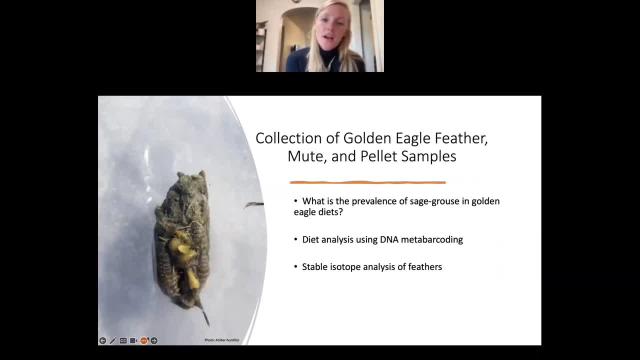 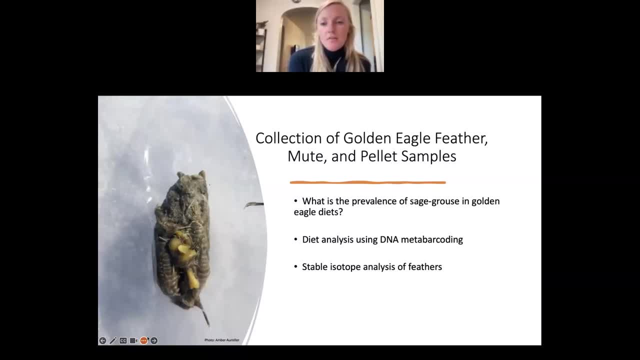 If you're not familiar, mute is the basically feces and urine combined, And this is to help me answer the question of the prevalence of sage-grouse in golden eagle diets. So I can do that by doing DNA metabarcoding of the pellet and mute samples and this 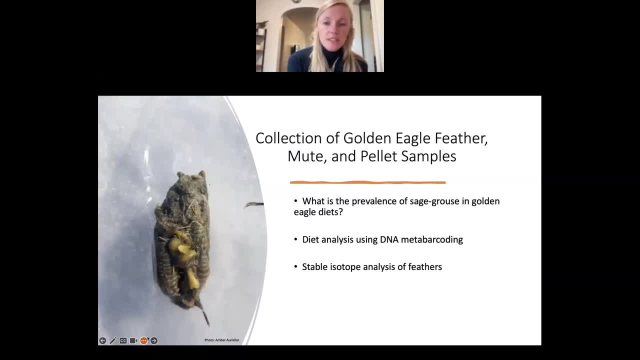 will look for the DNA of the orange and yellow생án of various prey species, And so I look for them, prey species, and from that I can get an idea of how many samples contained sage grouse DNA in them. And for feathers I can do stable isotope analysis to identify the origin of the feather. 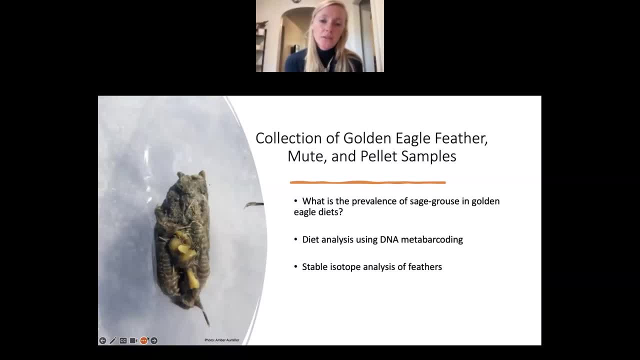 which will also help answer whether or not the golden eagles in the area are year-round residents or migratory eagles. And this photo here is a picture of a fresh pellet that I found underneath a power pole And it's kind of hard to see, but there's a sage grouse foot in there. 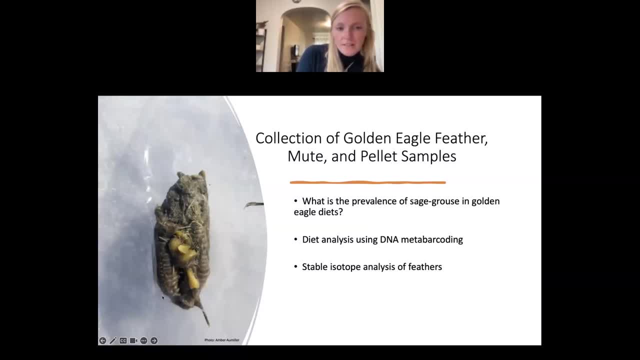 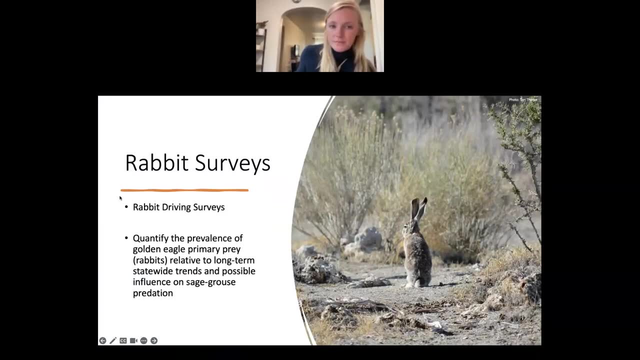 You can see the skin of the foot and then poking out of the top are the sage grouse nails. I'm also doing rabbit driving surveys, So these are conducted on the way to the LEC sites each morning and I'm hoping to quantify the prevalence of golden eagle. preys. I'm hoping to quantify the prevalence of golden eagle preys, So these are conducted on the way to the LEC sites each morning, and I'm hoping to quantify the prevalence of golden eagle preys, So these are conducted on the way to the LEC sites each morning, and I'm hoping to quantify the prevalence of golden eagle preys. 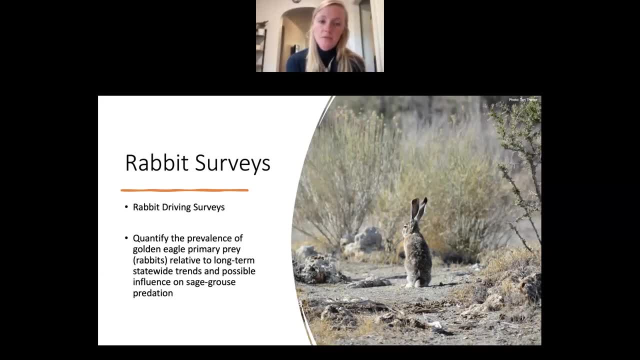 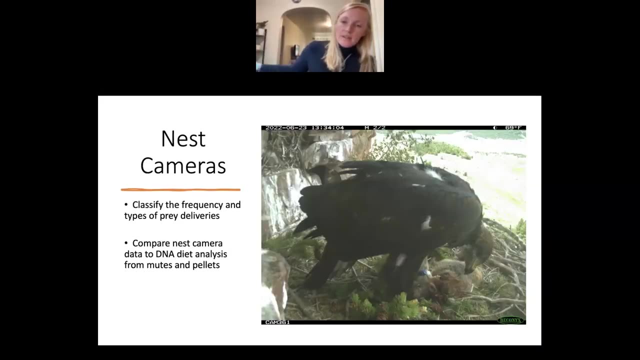 Relative to long-term statewide trends and possible influence on sage grouse predation. This will help me get a baseline understanding of prey abundance on Diamond Mountain as a whole. I'm also deploying nest cameras And this is to study the various types of prey delivered to the nests. 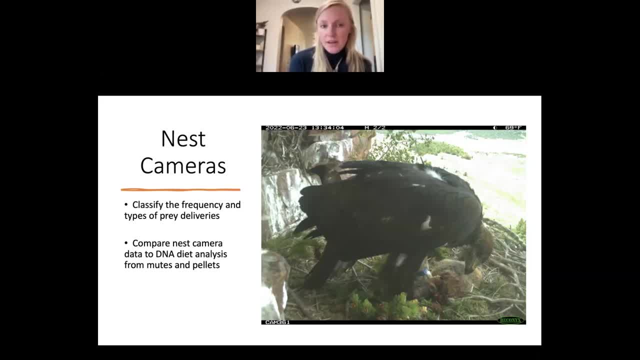 And I can use this camera data to classify frequency and types of prey delivered. And I'm hoping to compare what I see on the cameras to what I find for prey species in the DNA analysis of the pellets and the mutes. And unfortunately this year we only had one in use- golden eagle nest- that remained in use through the nesting period in the study area. 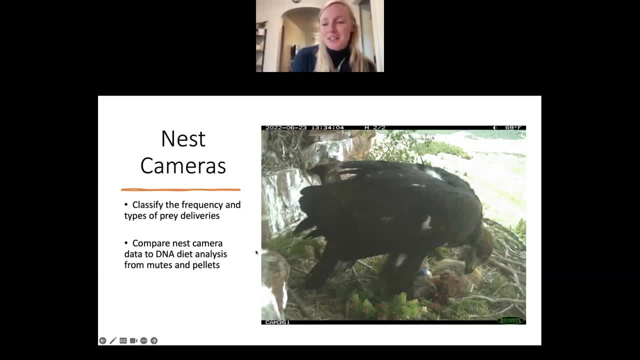 That was also accessible to repetitive use And this photo is from that nest And you can see that the nestling has a marmot that one of its parents delivered to the nest And you can also see the transmitter on the back of the eagle. 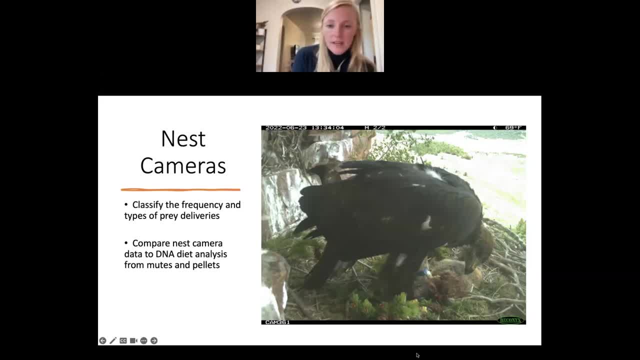 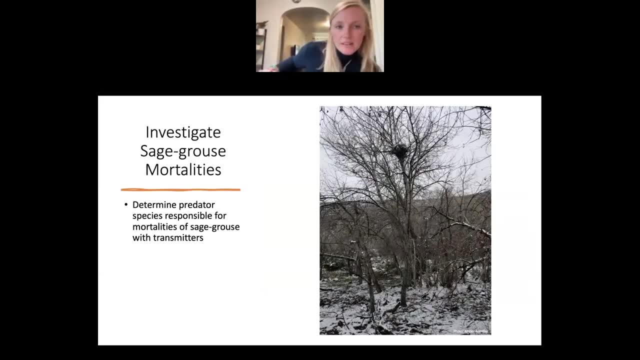 And it's color band that helps recite the individual. The last component of my study is investigating sage grouse mortalities. So some of the sage grouse in the study area have transmitters And when the transmitter is showing a mortality signal. 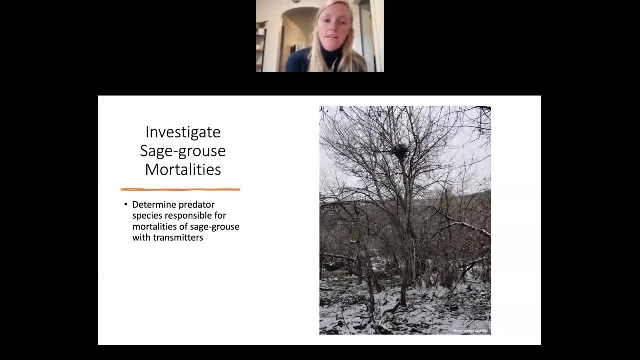 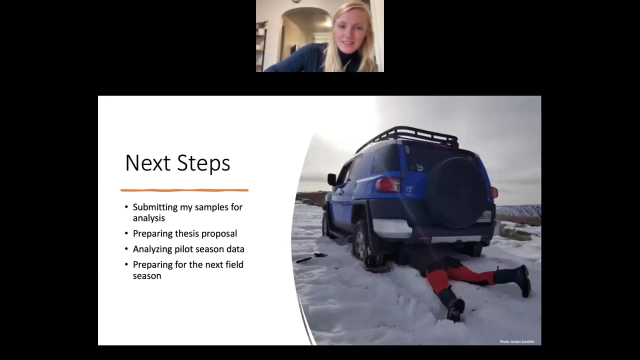 We can find the transmitter and hopefully find out why the sage grouse died. And this is a photo from an in use great horned owl nest that my technician found found and the sage-grouse transmitter is in that nest. So the next steps going forward are submitting all my samples for analysis, preparing my 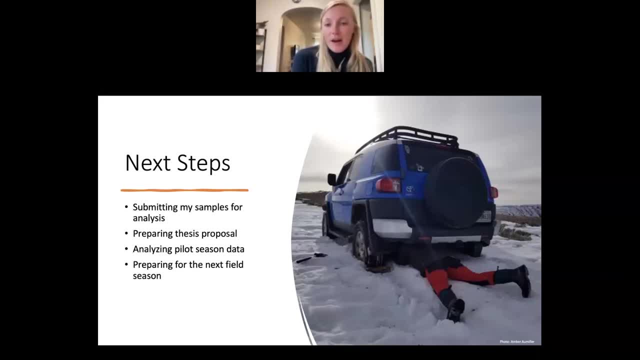 thesis proposal for grad school, analyzing my pilot season data and preparing for the next field season- And this photo is from early in the field season when a lot of the roads to the Lex were still covered in snow and I'm trying to dig out my car because we got it stuck. 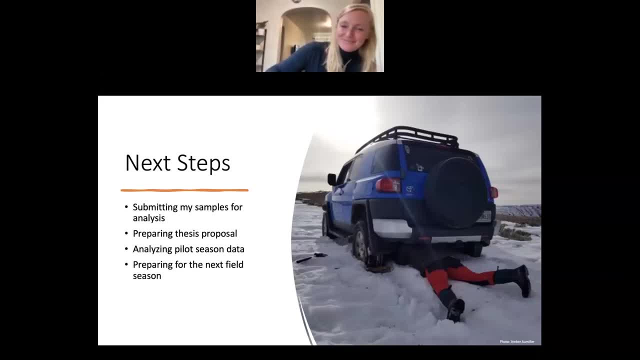 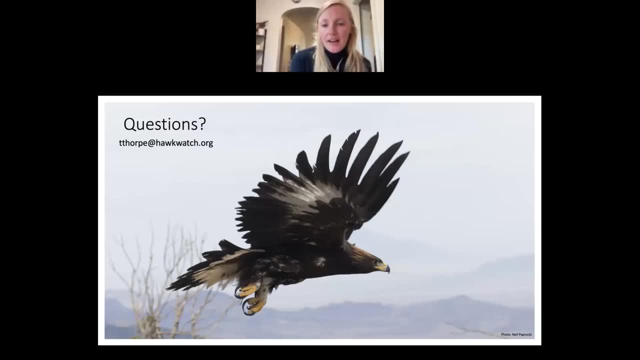 in the snow. Now I'll turn it back over to Sami and we'll answer questions from the chat at the end of Fidel's presentation. but if you don't get your question answered, feel free to email me at tthorpe, at hawkwatchorg. 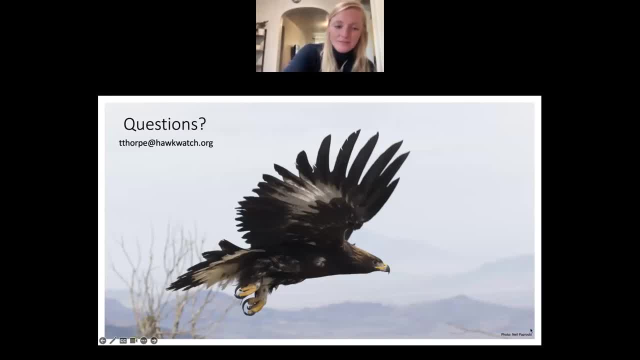 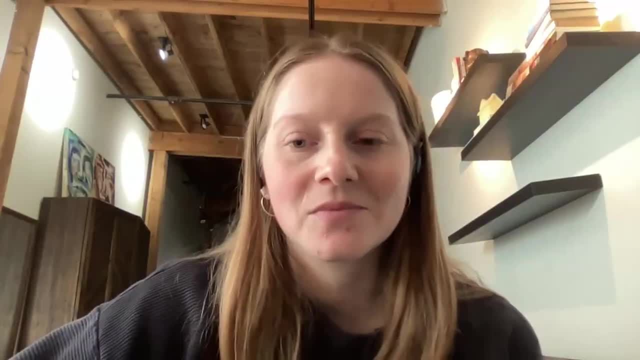 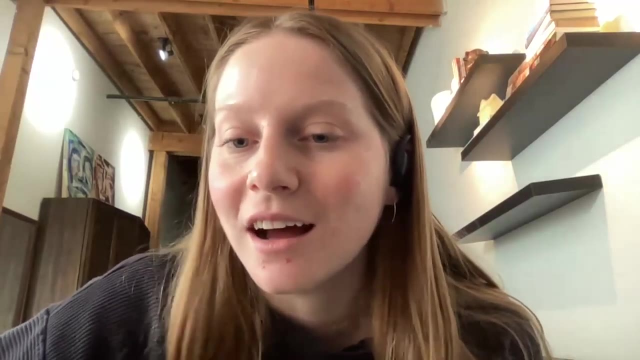 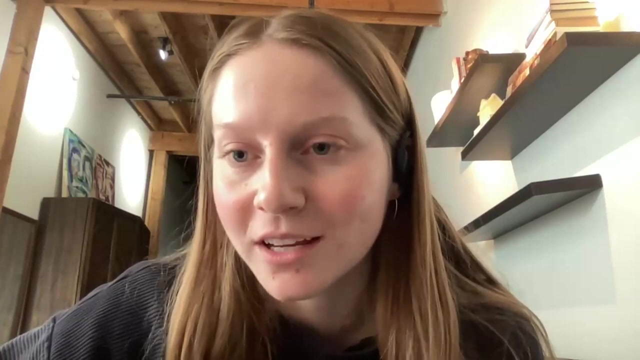 Thanks. Thank you, Tori. That was great. I'm excited to see what we find out throughout your masters. So, Tori, I have a question for you in the chat, and they ask if you've observed more resident eagles predating on the sage-grouse or if you've seen more younger birds doing. 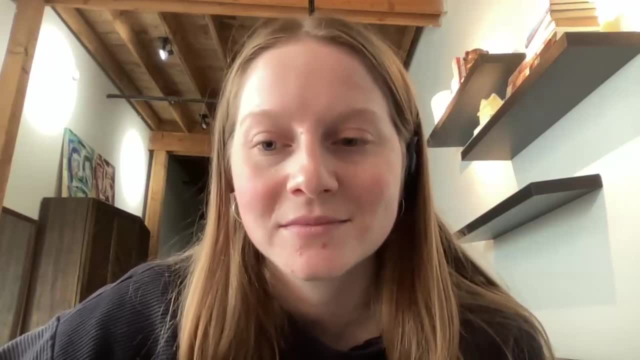 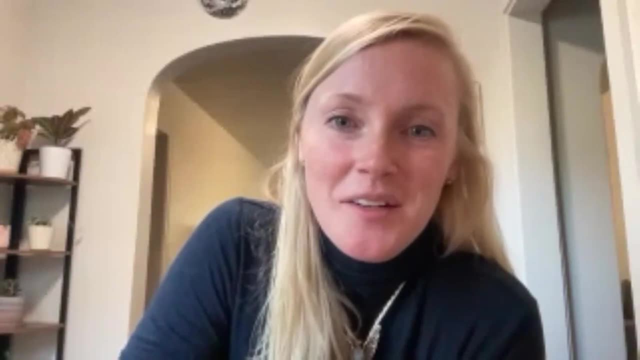 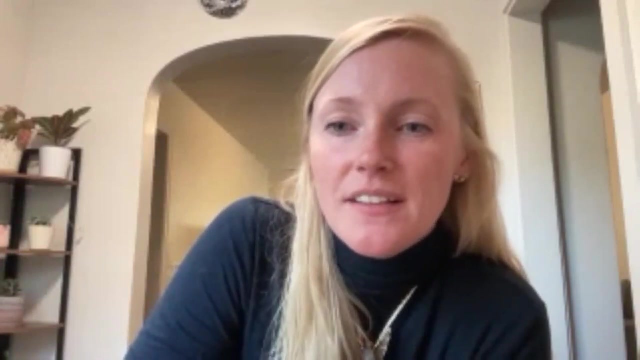 it in your first season of fieldwork. In the first season we actually never observed a successful predation from eagles on the grouse. It did seem that younger eagles attempted more, but I'm hoping to find a lot more information in the next two years of fieldwork on whether or not most of the eagles hanging around are. 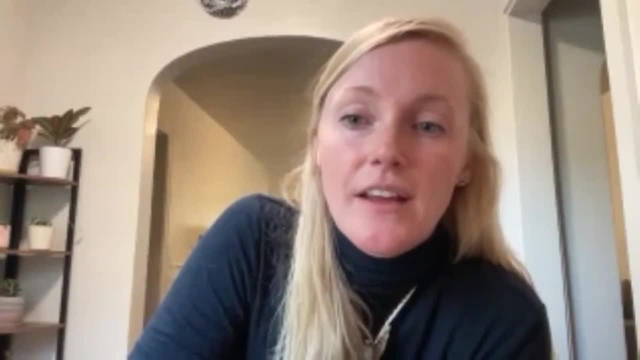 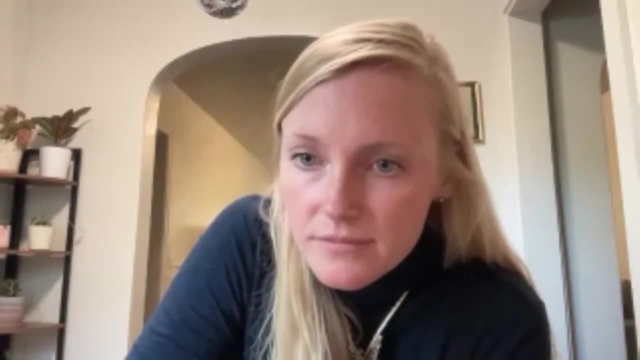 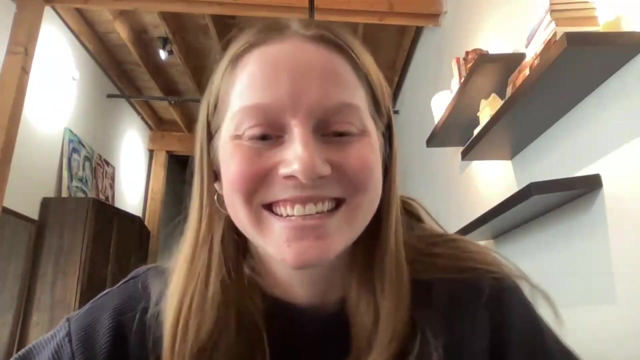 migratory eagles or year-round residents, and the age as well. So what's your guess, Tori? Is it working? Yes, We hear you. Okay, Perfect timing. Excellent. Still seeing my screen? I'm not seeing it yet. 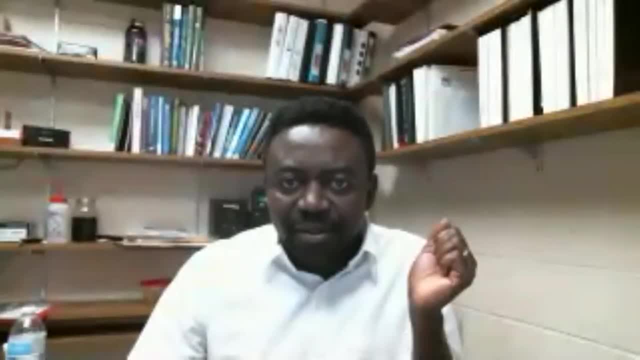 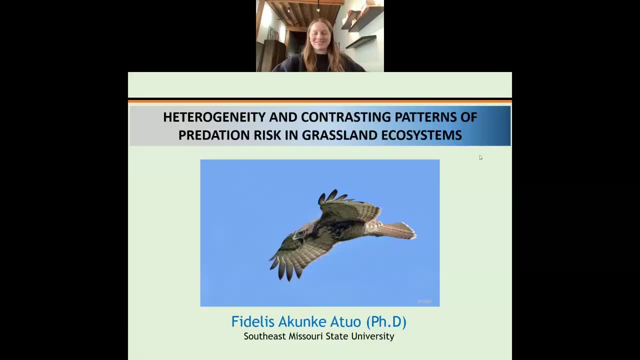 There we go. You're ready to go? Okay, Okay, guys, sorry about all the technical difficulties. My name is Fidel Atuo and I'll be sharing with you here the work I did several years back, So this is not as recent as Tori's work. 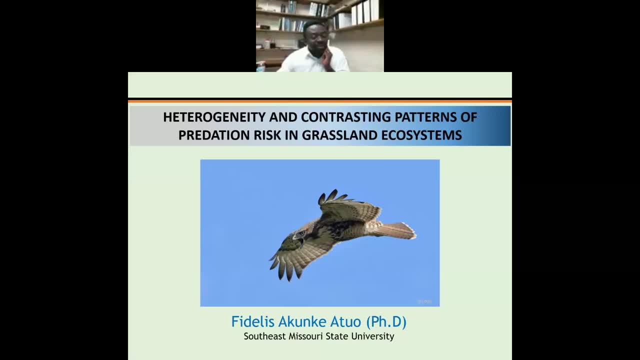 So mine is a little bit older, So it will be. I don't think many things have changed since I completed this work, but I've not been in touch to check it out, So I'm going to talk about how habitat complexity might affect protection risks for grassland. 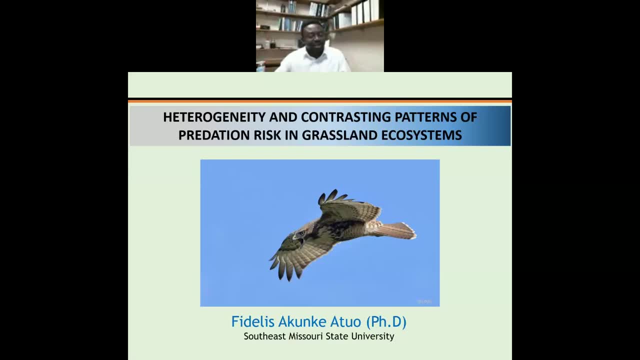 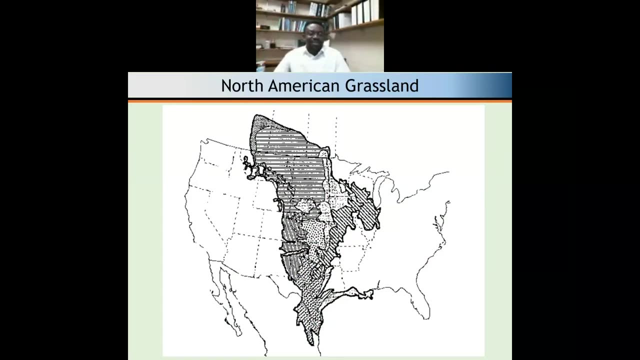 obligates, like the sage grass that Tori just showed. So we know That historically, most of these areas within the central United States here were just grasslands, So there were huge open grasslands and we've lost much of that due to so many anthropogenic. 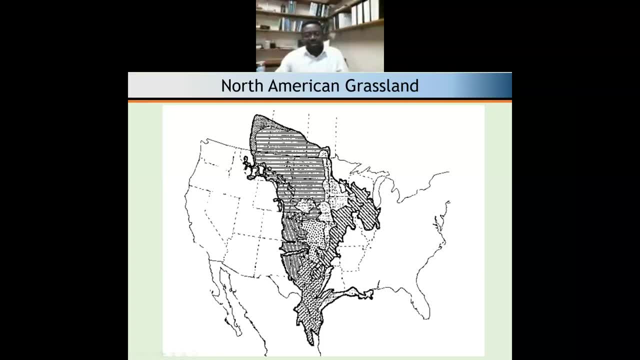 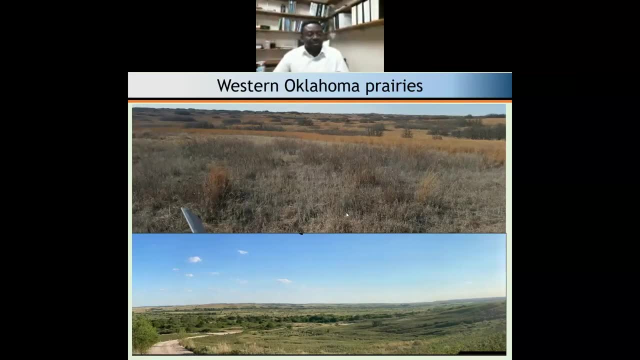 disturbances. I will talk about them here in a minute. but if you were to look at grasslands- mostly like the ones we have here, The ones we have in Western Oklahoma- they look like they are just open plains, large areas of grasslands that are preferred by grassland obligates, mostly, I would say, birds. 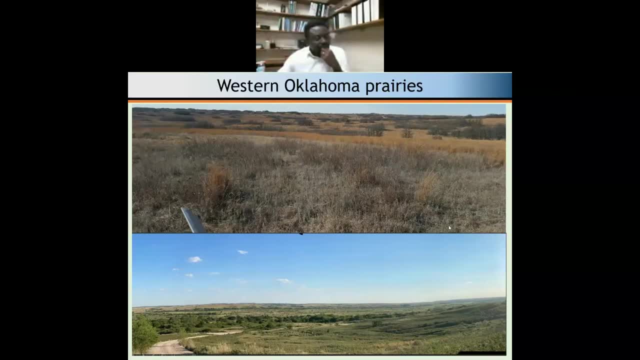 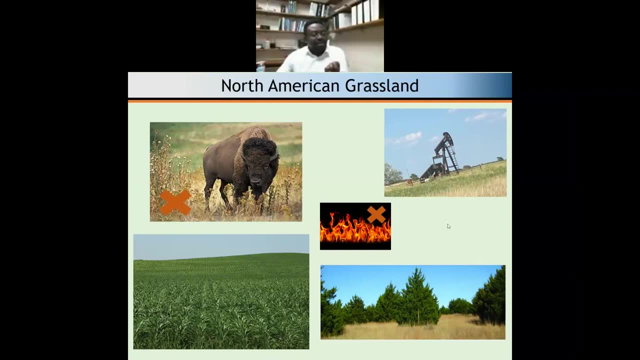 that I'm going to focus on today, So the things that have really affected these grasslands, Things like massive agriculture that comforts grassland ecosystems to farms, or here we see woody encroachment, So it could be just the encroachment of woody vegetation. 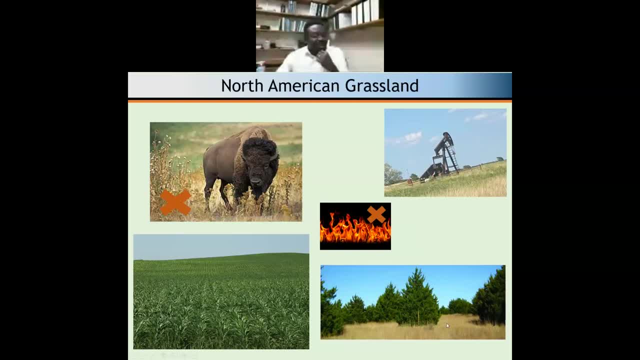 Remember, like Tori said, most of these areas evolved not to have structures, So the presence of these structures really transformed grassland Into something else, or maybe just oil explorations like the ones we have here. Grassland ecosystems are traditionally maintained by disturbance regimes like fire and grazing. 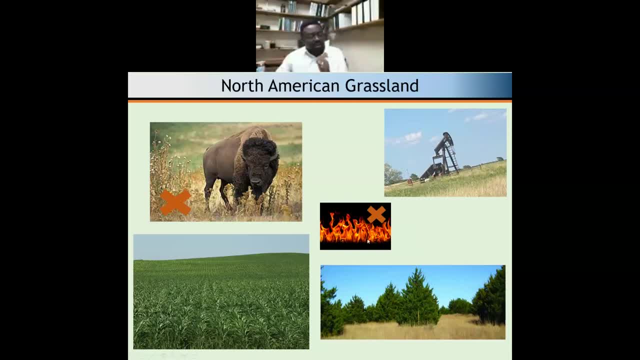 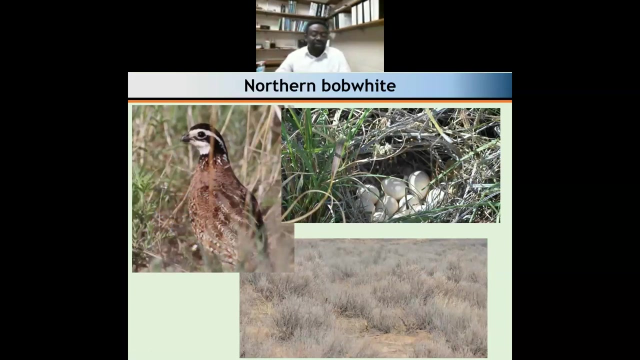 And we've seen a drastic reduction in this stuff as well. So the absence of fire and grazing might affect the way grassland functions and the ecosystem's services that they provide. So for grassland birds like quail, which is a little bit smaller than sage grass here, 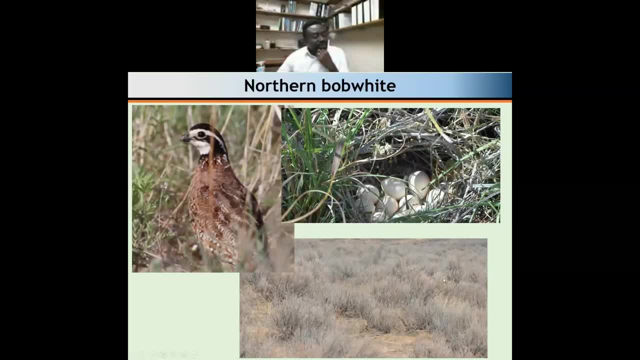 which again what we have in Oklahoma. they require large areas of grassland to reproduce, even though they require some variability with the environment. So, for example, if you look at this one, here We're doing this grassland ecosystem. It is important today that grasslands are maintained at large patches such that they 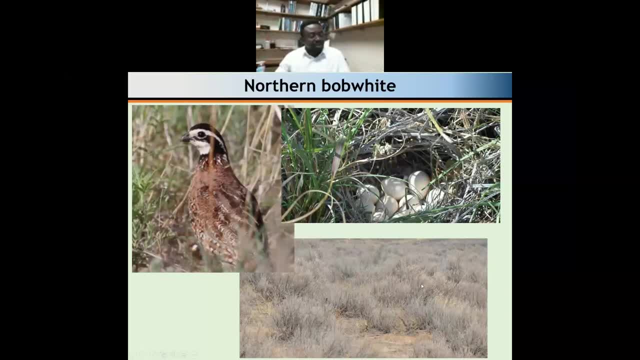 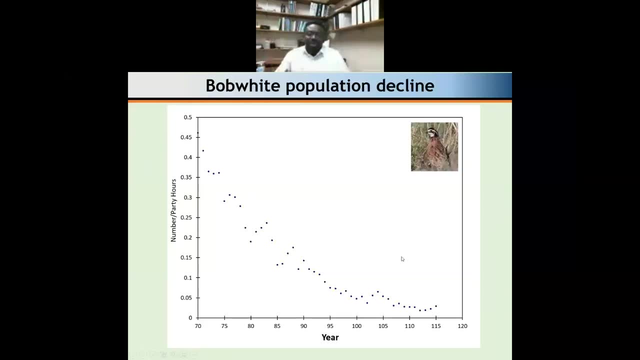 can forage, have their reproductive activities, lay their nests and raise their young. Something that we've noticed in the past several years is that populations of most of these grassland obliquates have been degraded. So this is the example of this. 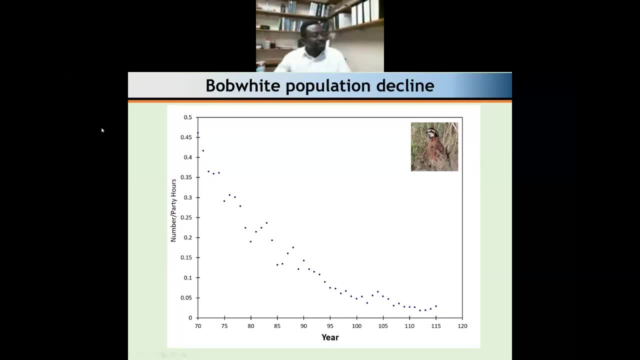 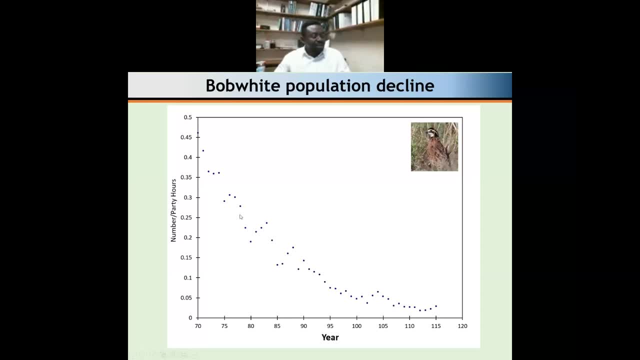 in the populations of bobwhite quail in the last several decades. So several reasons can be attributed to this decline, Like I've showed from the beginning: the loss of grassland ecosystem due to woody encroachments, lack of fire in grassland ecosystems. 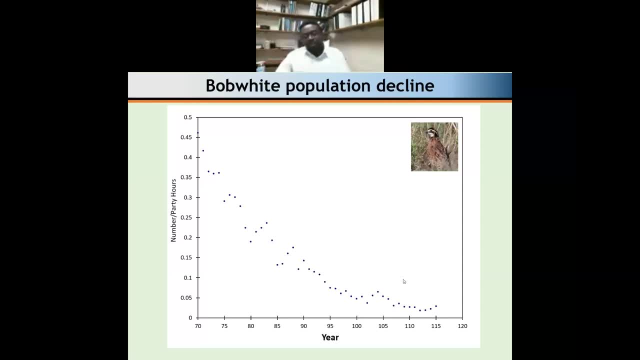 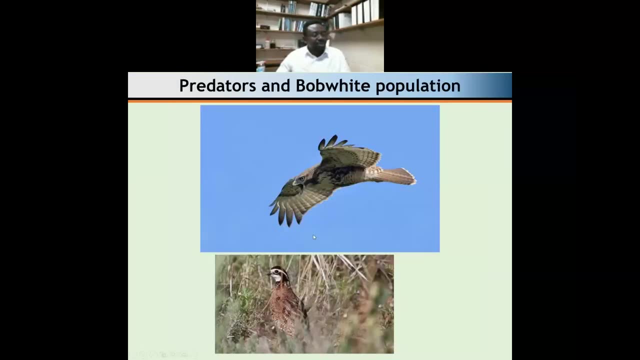 or lack of grazing. all of these contribute to loss in grassland ecosystems and they affect quail. But something that we've not really paid much attention to, or, in the other hands, have been exaggerated, is the impact that predators can have on birds like quail. 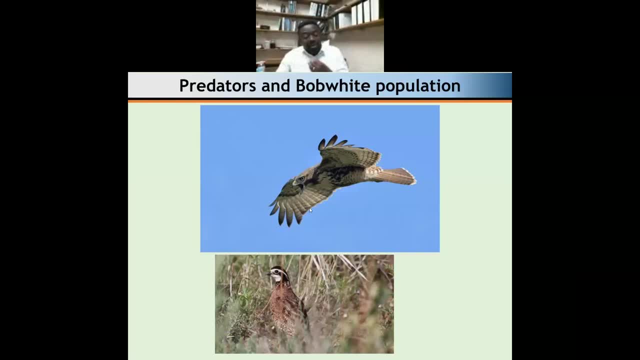 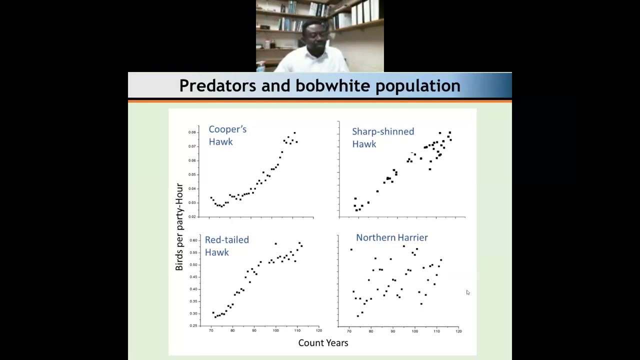 So in this study I tried to explore how predators can directly or indirectly impact quail populations. Again we go back to Tori's presentation about raptors population. It's true, over the years we've seen huge decline in raptor populations prior to the 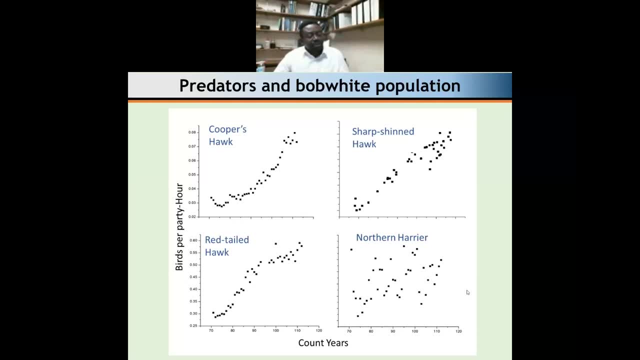 the protection that raptors received. So when we stop all the bounties on raptors and again coupled with the ban on DDT, we've seen steady population growth for most raptors. So looking at raptors like Cooper's hawk, 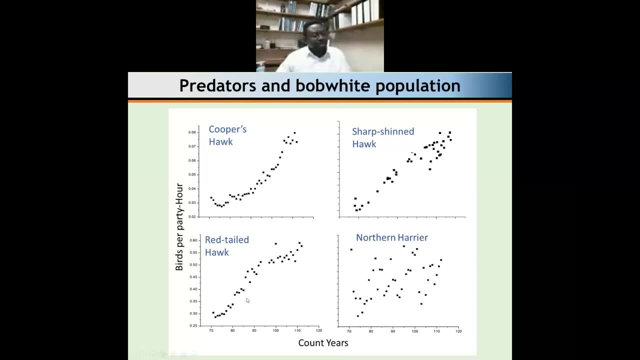 Shamshafshin hawk or red-tailed hawk- they've all witnessed a steady population growth. So for most people they're not going to be able to survive. So for most people they're not going to survive. So for most people they're not going to survive. 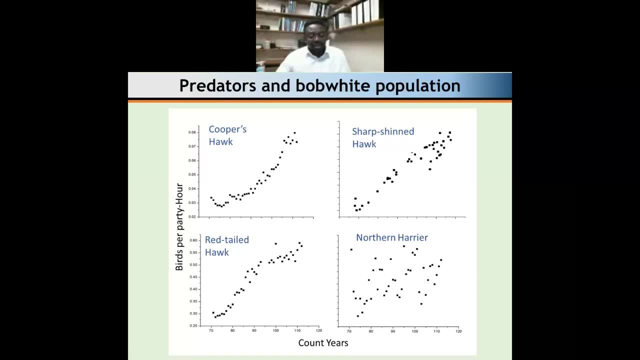 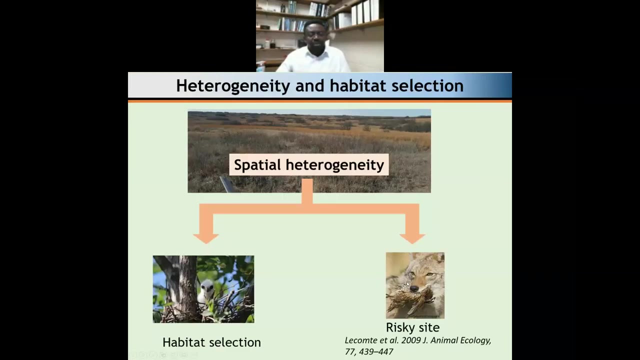 So for most people, it is so easy to incriminate raptors as a key driver of population declines, as a key driver of population declines in vulnerable prey species like Bob white quail. So the question I choose to ask in this research that I'm sharing with you is: 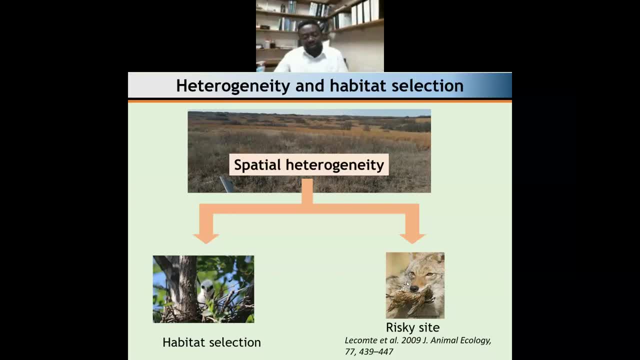 how does raptor predation really impact quail population? How does raptor predation really impact quail population? How does raptor predation really impact quail in the face of changes in grassland habitat structure? So I will call this heterogeneity at this point. 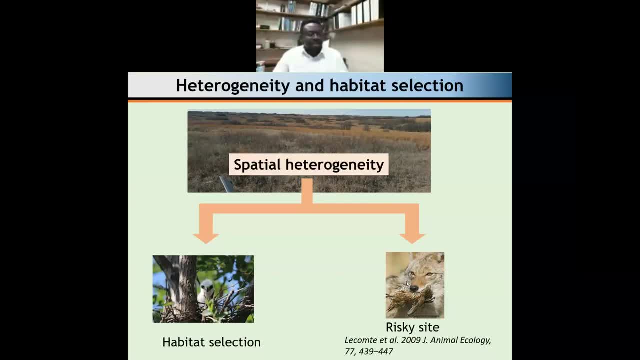 but basically it is just habitat complexity, mediating the impact that predators might have on prey species. Indeed, when we manage habitats for biodiversity, we often do this. We often do this to increase heterogeneity, So heterogeneity is a great thing to do. 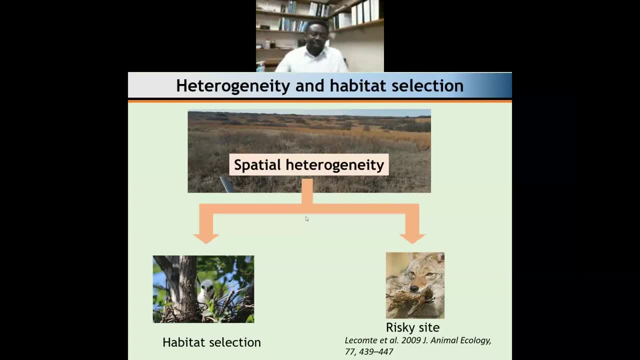 in all habitat management But again, depending on the scale of heterogeneity, it might be a great support for habitat selection. it might be a great support for habitat selection or might just create risky sites for some vulnerable species, And several studies have documented this. 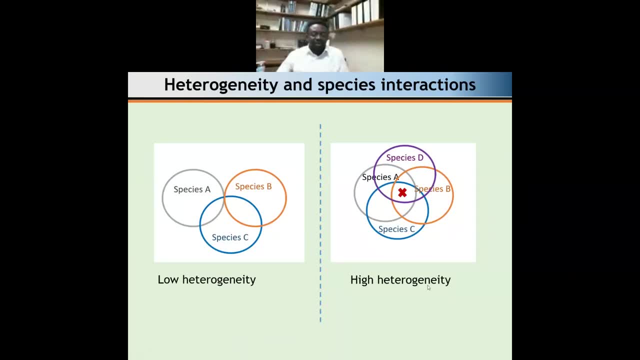 So I will show this a little bit using our concept of niche partitioning in ecology. So let's say we have three areas. We have these areas that are colored differently in this part of the presentation or the slides rather, So let's say, species A prefer this area. 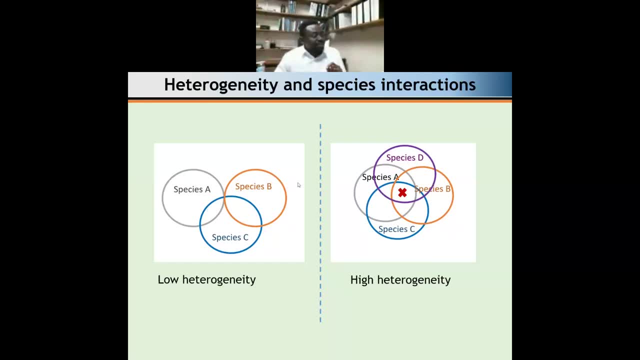 So let's say species A prefer this area. So let's say species A prefer this area, This area that is in gray, species B prefer that area in orange and species C prefer that area in blue. And we have sufficient large patches of each of these areas. 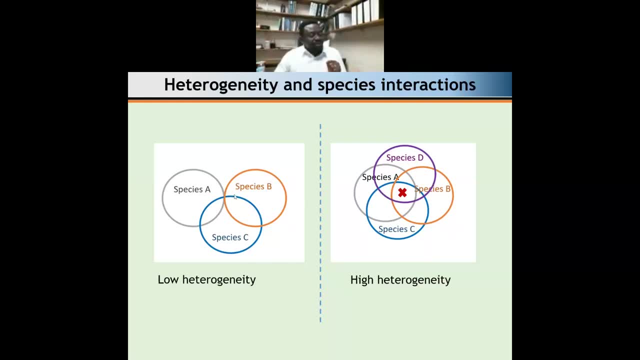 Then there will be little need for these species to come in contact and in conflict. But if we change this patch structure such that we bring little patches of each of these mixed together, then we put all of these species in close competitive proximity And what that happened is that as many species 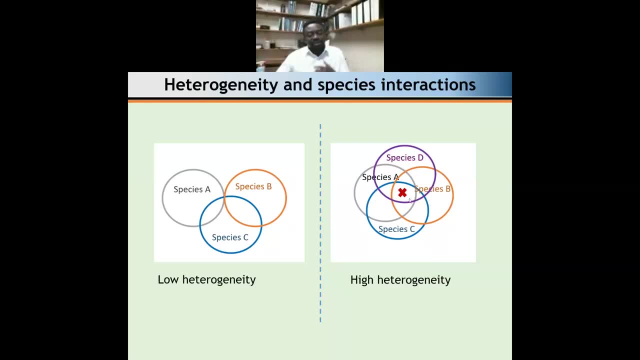 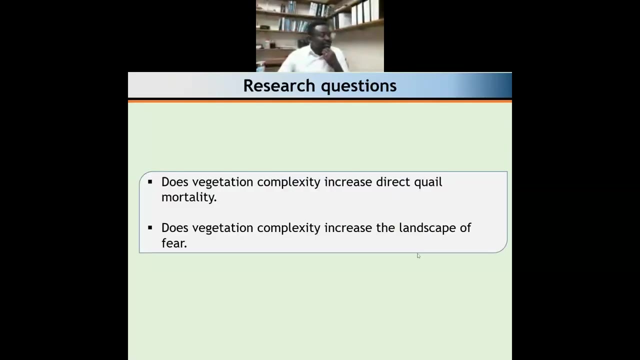 try to compete for limited resources, there had to be intense pressure on some vulnerable species that have not evolved adaptations to deal with these multiple predators. to deal with these multiple predators. to deal with these multiple predators. So here I'm asking simple questions like: 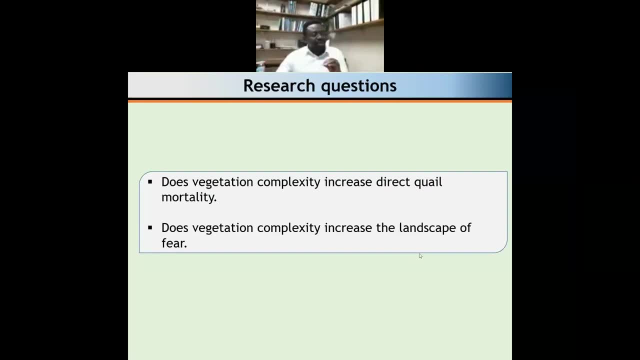 does vegetation complexity really increase the direct impact that predators might have on prey species like quail, that predators might have on prey species like quail, And if this habitat complexity also creates some form of fear? And if this habitat complexity also creates some form of fear. 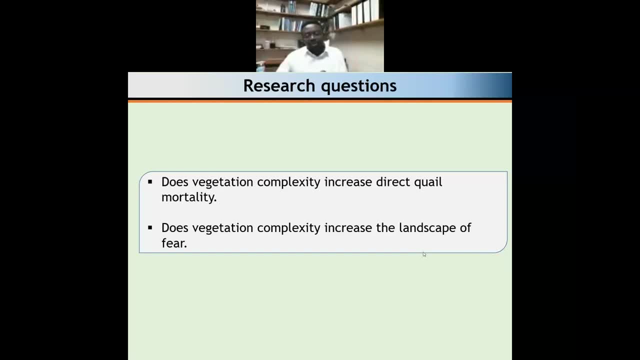 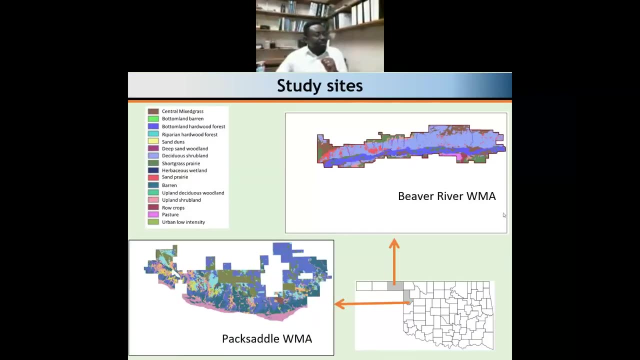 which would be indirect impact of predation on prey such that it affects their habitat, such that it affects their habitat, such that it affects their habitat. So this work I did at two wildlife management areas in Western Oklahoma, so Pack, Saddle and Beaver Wildlife Management Areas. 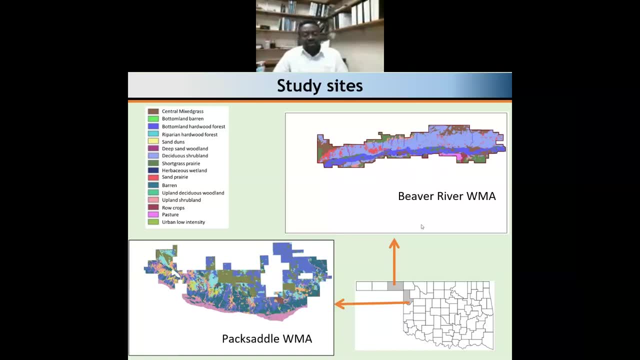 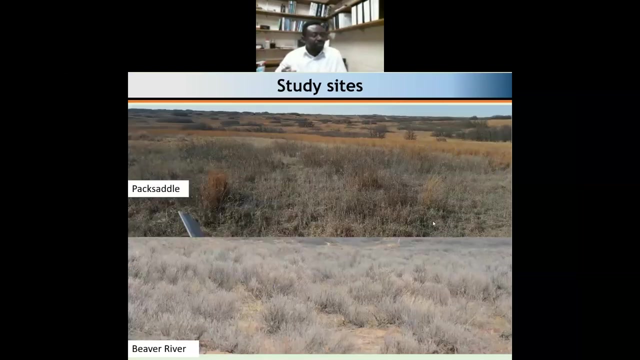 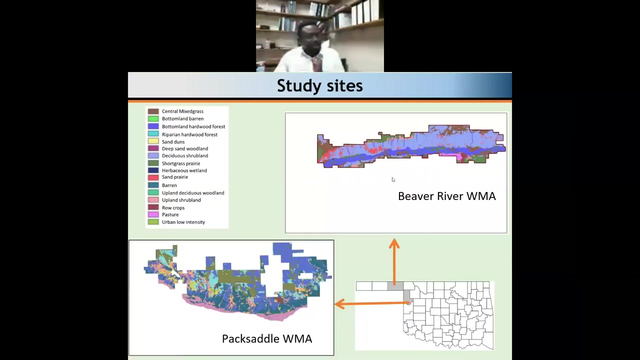 Both areas are managed by the Oklahoma Department of Wildlife Conservation, mostly to increase populations of quail and maybe other fauna species, But the main focus on each of these wildlife management areas is to increase quail populations. is to increase quail populations, Okay. so if you look at these images, 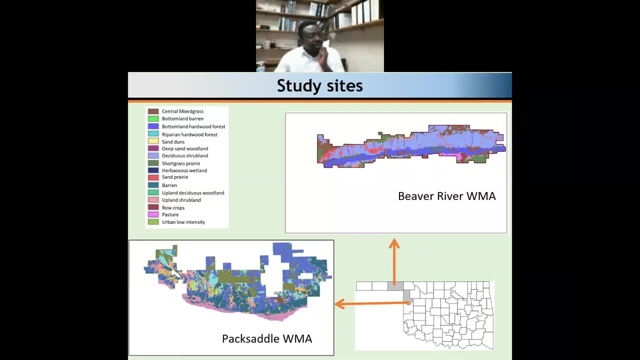 you will see a vegetation map of Beaver River and that of Pack Saddle. Something that should jump out to you right away is that Pack Saddle- Something that should jump out to you right away- is that Pack Saddle appears to have these little complex colors. 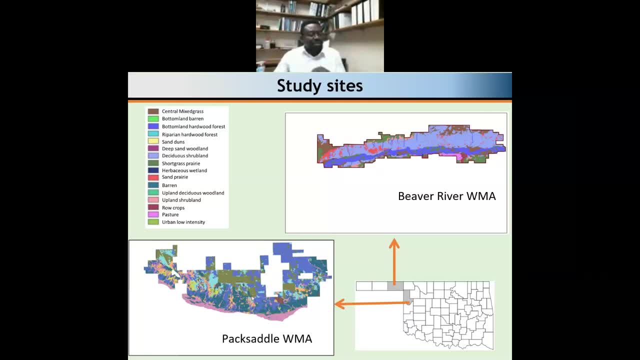 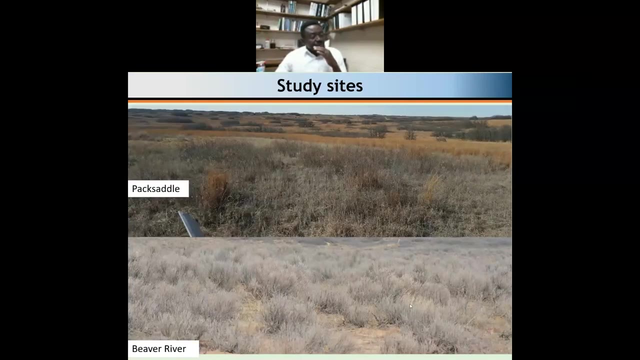 that shows a landscape with tiny patches of different vegetation, While Beaver River appears to have these large areas of unique vegetation types. So if you were to visit this landscape, this is what you will see. So Beaver River- this is a huge area with less complexity. 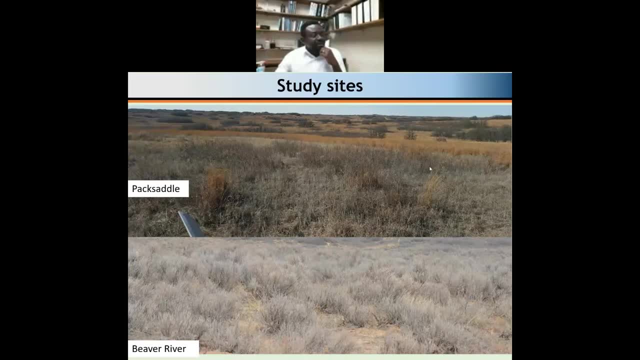 Pack Saddle, another huge area, but this time around with a lot of that woody vegetation sometimes crossed out of there. all scattered in upland areas of the management. all scattered in upland areas of the management, the wildlife management area. 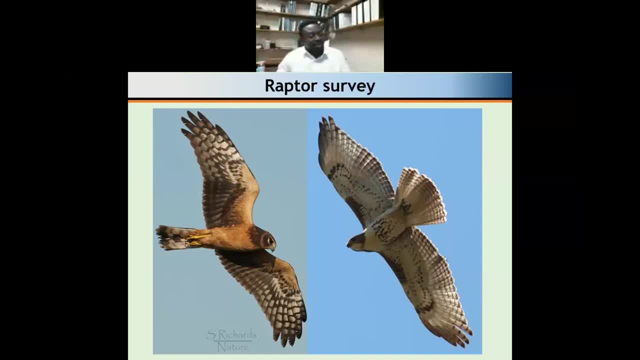 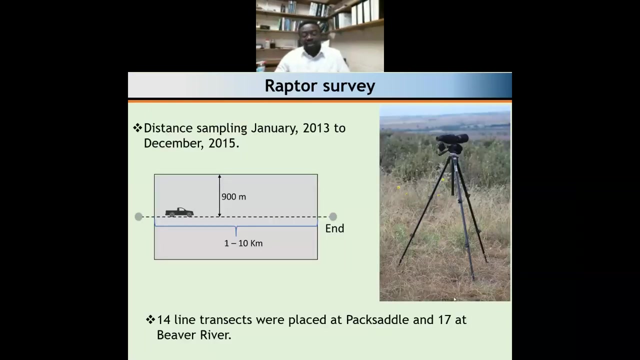 Several predators or several raptors would take quail, But in this presentation I'm just going to focus on two species like the red-tailed hawk and the northern harrier. So first what I did was to go out and estimate the population. 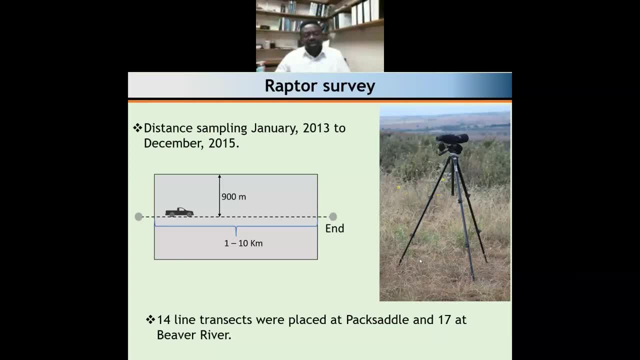 or the abundance of these predators on the landscape and see if they have any impact on quail. So I drove around transit lines that I started. So I drove around transit lines that I started in this area and counted all the raptors that I saw. 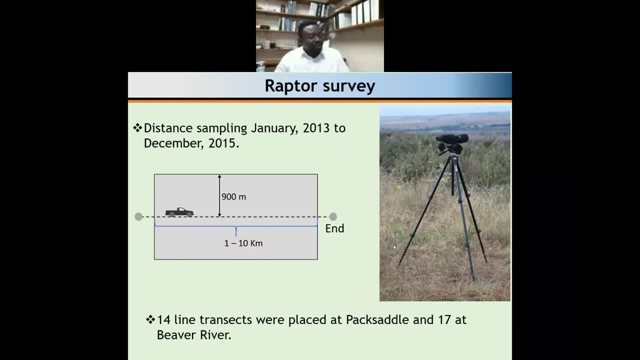 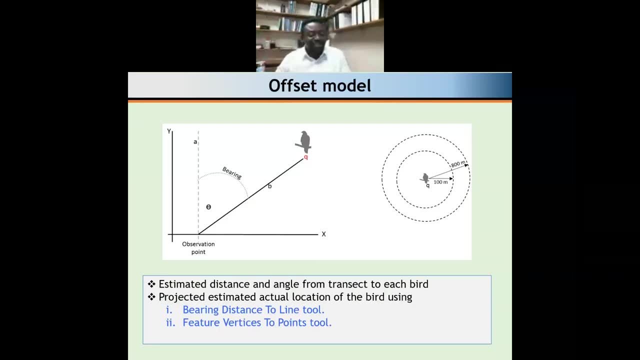 with focus on red-tailed hawks and northern harriers. I didn't have all the resources that Tori has right now, so I couldn't get all the fancy equipment that we needed for this work, So I couldn't trap raptors and put transmitters on them. 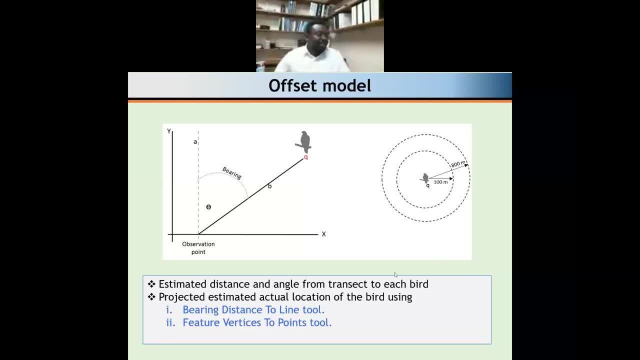 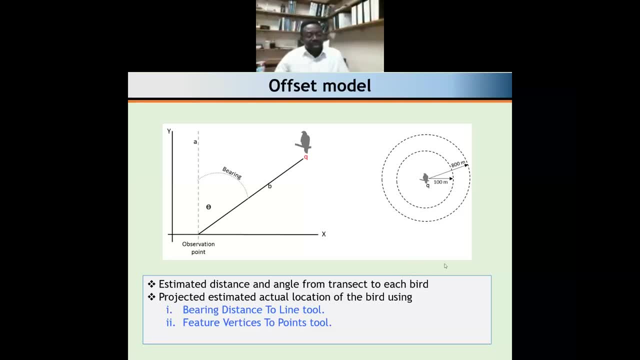 and wherever I sighted a raptor, I would mark tech GPS coordinates representing the location of that raptor. So, as you would expect, those GPS locations- because they were taken by me from the comfort of my truck- would not represent the actual location of the bird. 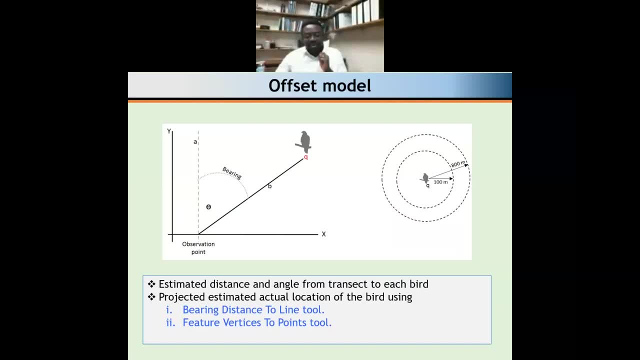 as of the time it was sighted. as of the time it was sighted. Rather, they will represent my location at the time I sighted the bird. So I needed to figure a way of moving this point to the actual location where the birds were sighted. 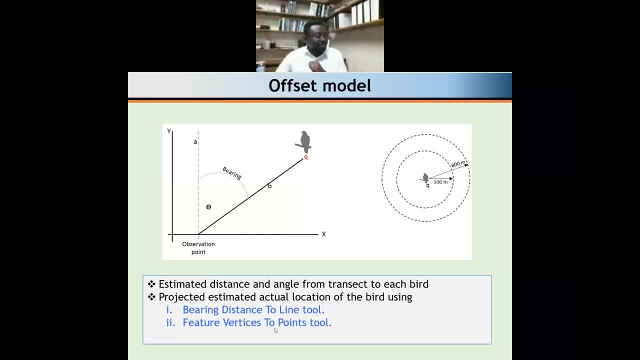 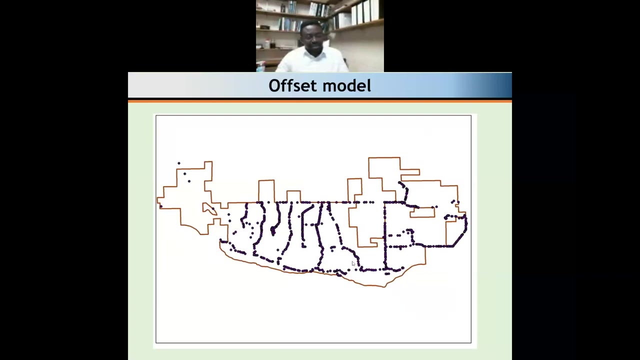 So I did that using some of these cool GIS tools that are available to anyone that is able to use GIS. So with these tools- I was able to use GIS tools that are available to anyone that is able to use GIS- I was able to move points that I collected along the transit line. 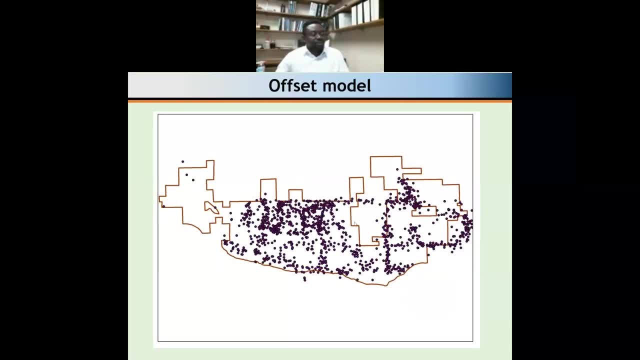 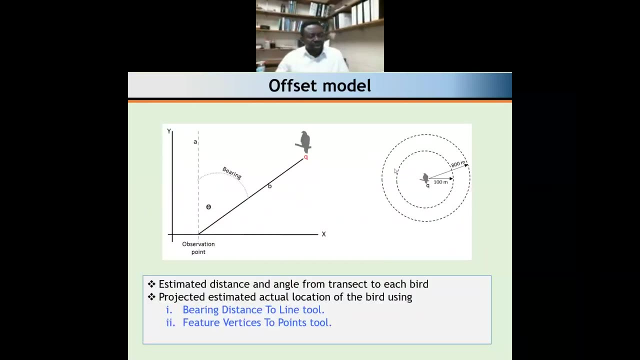 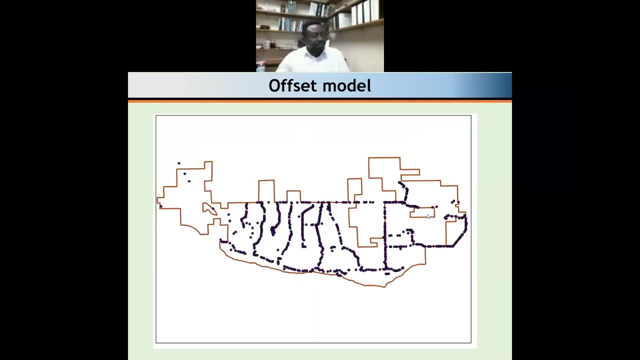 like demonstrated here, to exact locations where birds were found. So now the points represent birds locations and not my location. And once I was able to do that, I then put buffers around each point, at different spatial scales to estimate vegetation cover. at different spatial scales to estimate vegetation cover. 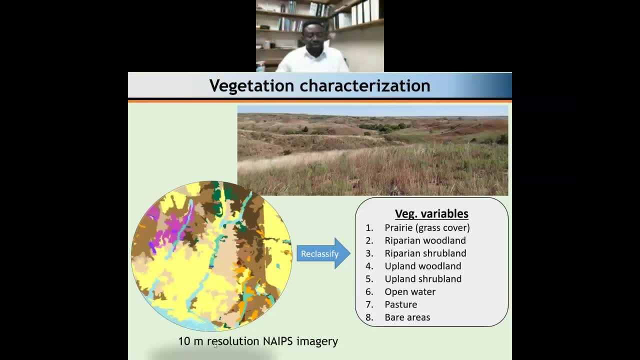 Luckily we were able to obtain this 10-meter resolution neat image of the land cover map of these two areas. neat image of the land cover map of these two areas. So once we had these maps, we put buffers around locations that represented bird use. 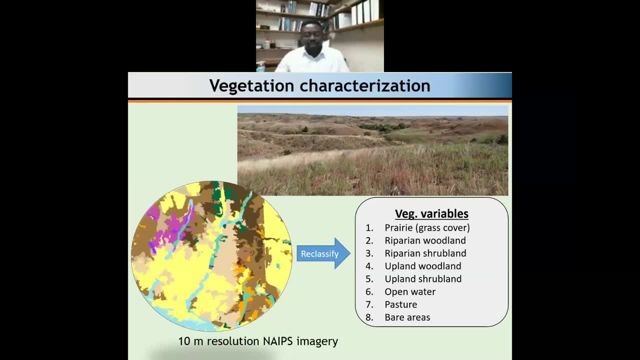 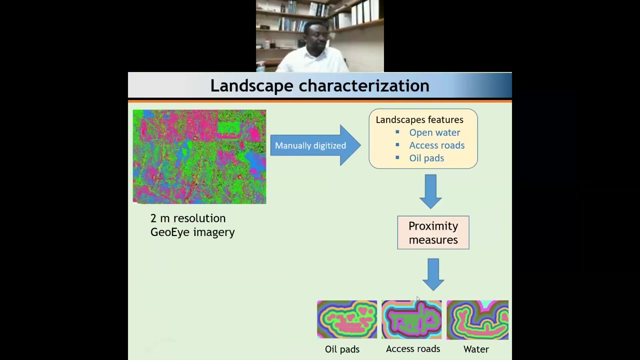 we put buffers around locations that represented bird use and extract vegetation that occur within those buffers and extract vegetation that occur within those buffers. So for most vegetation cover I was able to reclassify those into about eight different cover types, into about eight different cover types. 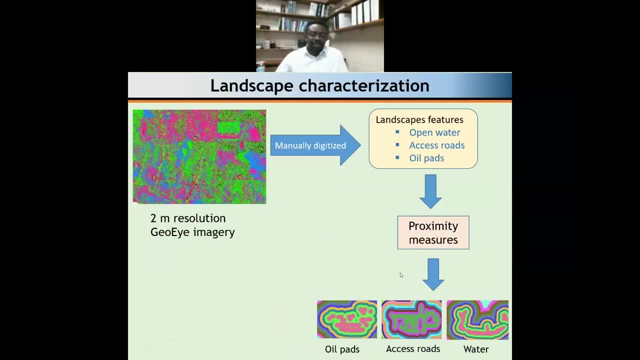 Sometimes organisms could select an area not just based on what the area holds, but based on its proximity to some other resources, or its proximity away from dangerous resources or its proximity away from dangerous resources. So to help me do that, we obtained this really fine scale. 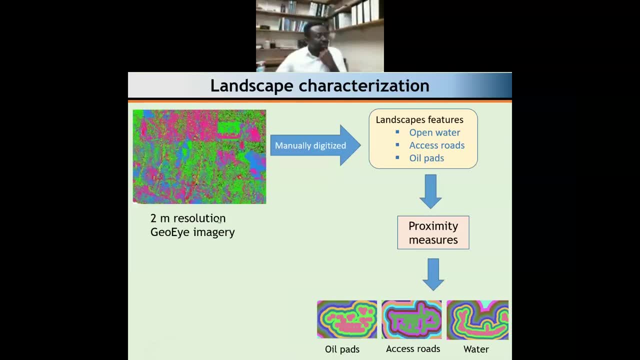 two-meter resolution image and then, using that, identified areas that were open, water access, road, oil, pines- and calculated or developed something that we'll call files of proximity. So I looked at, developed proximity and then I collected a lot of rasters from these images. 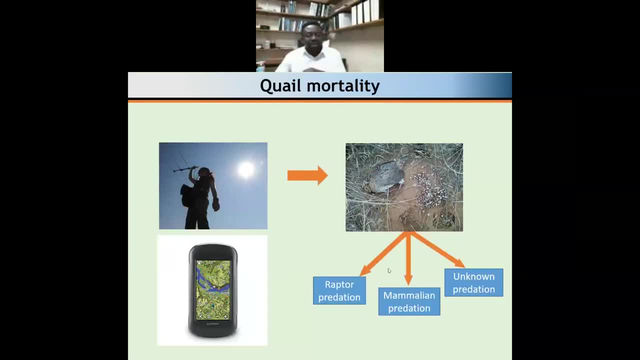 and collected a lot of rasters from these images. Okay, so that was a quick review of how I collected raptor data. The next thing was to find out where quail were dying. The next thing was to find out where quail were dying. 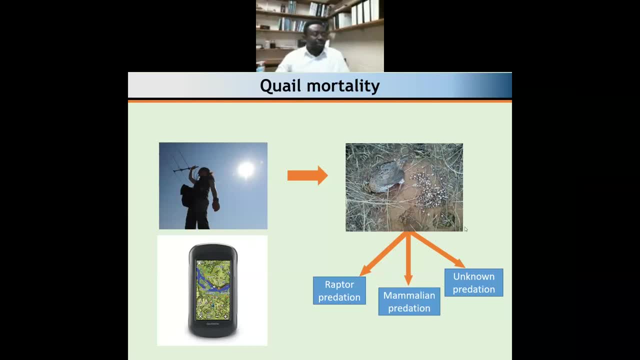 and areas that quail were utilizing. So to do that, we got other graduate students that. we got other graduate students that had trapped quail, put transmitters on them and we're tracking them. So we collaborated with them to find out locations. 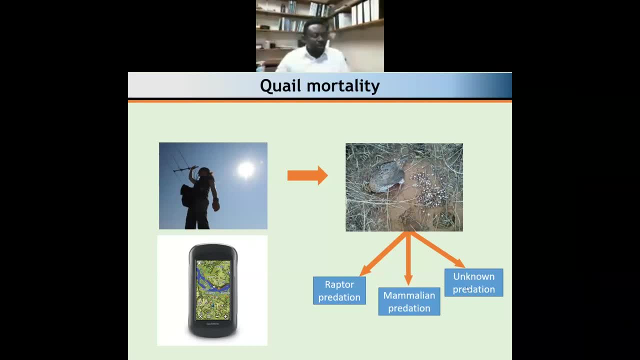 where mortality, where mortality were occurring. So they gave us locations of all areas that they lost quail And those areas. we also worked with them to identify the, the corporates, I will say that was responsible for that mortality. that was responsible for that mortality. 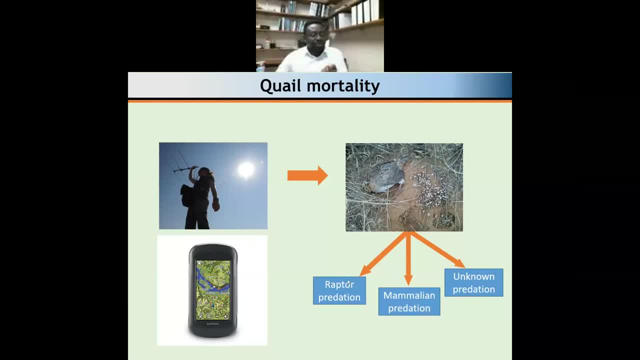 What was if a bird died through vitamin, if it was due to raptor predation, mammalian predation or simply an unknown predation event? So we collected all of those data and we're able to correlate them with raptor abundance. 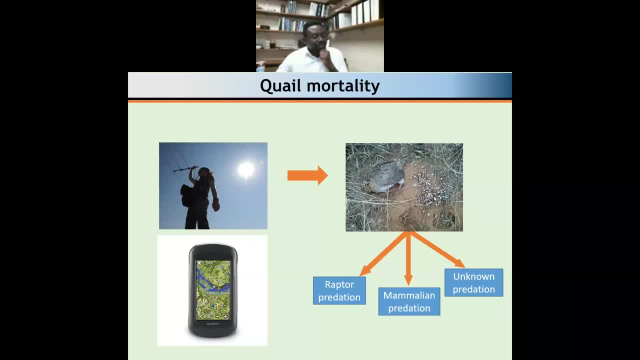 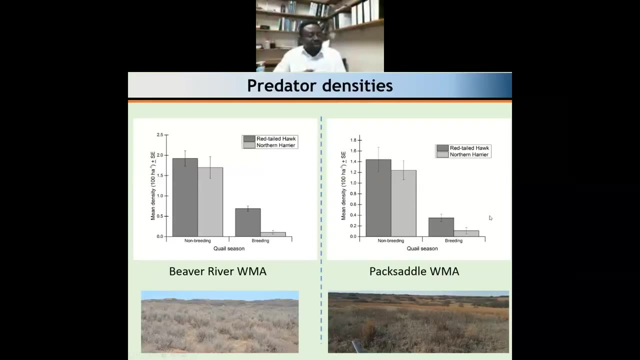 and habitat use. So those some results from that study. Well, the first thing we were interested in was to look at raptor populations And to do that we calculated raptor densities across these two ecosystems, or these landscapes. So again, remember, I showed you those images of Beaver River. 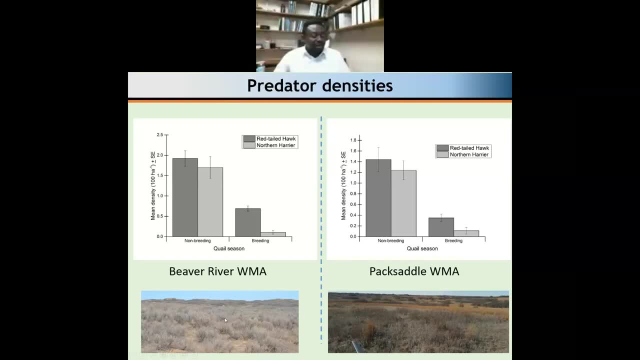 which is a more open area, traditional grassland ecosystem with less woody encroachment, and then Pikesaddle with that complexity, What we saw was that, in terms of population density, we had way more densities of raptors, specifically red-tailed hawks and northern harriers. 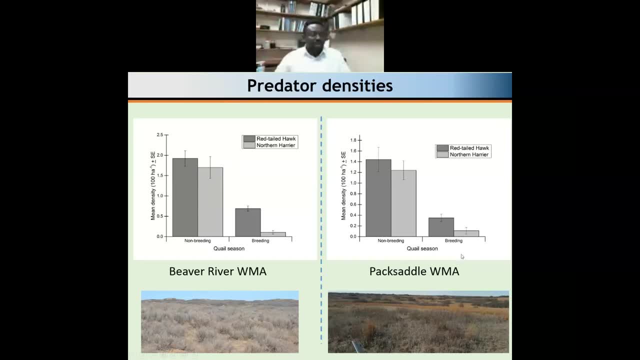 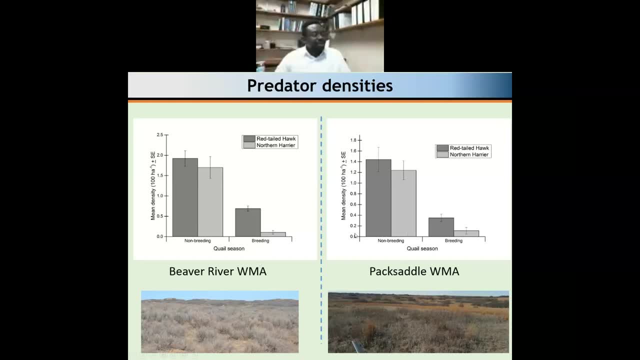 lies in a migration flyway where most raptors are overwintering during the winter and living back at the end of the winter season. So we had generally more abundance of these raptors. So we had generally more abundance of these raptors at Beaver River compared to Pikesaddle. 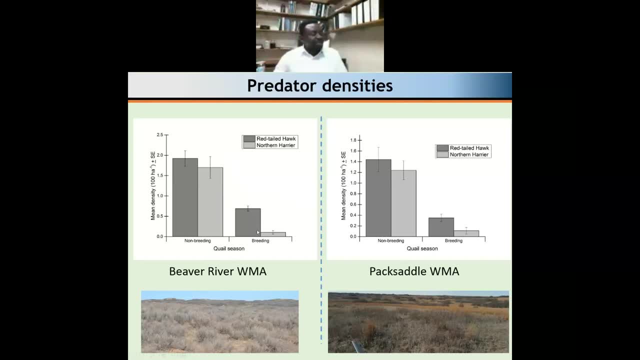 at Beaver River compared to Pikesaddle. And of course, because we are down south, we expect that in the winter that abundance will be way higher compared to the spring and summer, So that of course will correlate with the non-breeding season of quail. 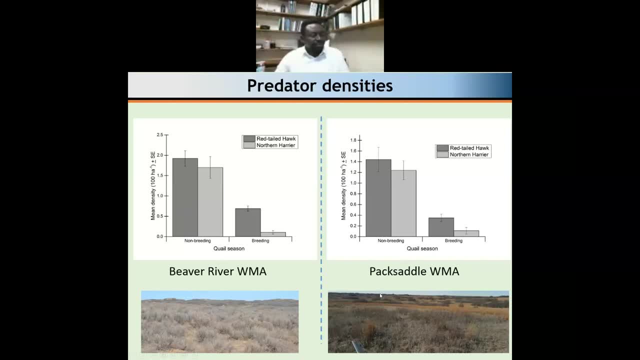 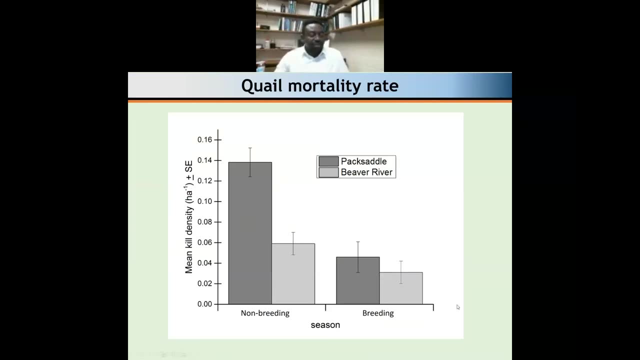 which is also the non-breeding season of these raptors. However, when we looked at mortality rates, However, when we looked at mortality rates, However, when we looked at mortality rates in these two wildlife management areas, we see a huge, significant difference. 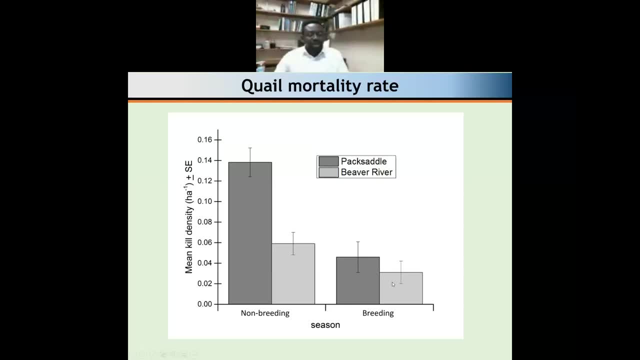 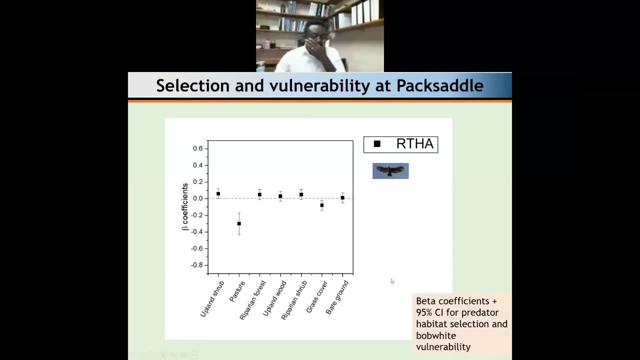 between Pikesaddle and Beaver River. Although we had a lot of raptors at Beaver River, mortality was way higher at Pikesaddle than Beaver River, which is less complex. So we decided to zoom in a little bit to look at the 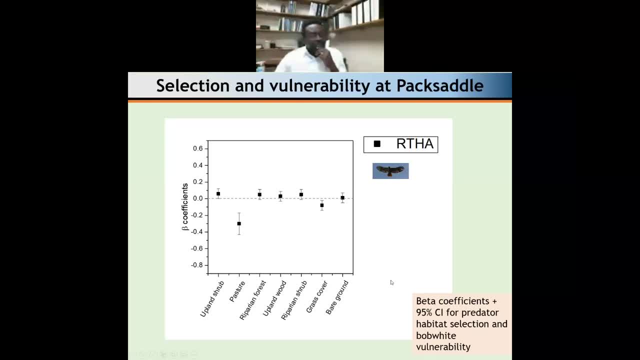 sort of areas that raptors were selecting first and see if those areas correlated with areas that we were seeing mortality rates for quail. So we did a simple analysis, something they will call resource selection function, but what that simply means is a regression analysis. 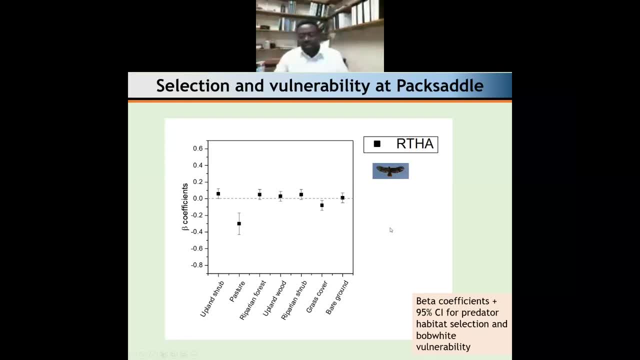 So it's a logistic regression analysis. So it's a logistic regression analysis, but what that simply means is a regression analysis with binary outcomes. So here we'll present the results of those analysis as they relate to yields. Now the dotted line in the middle of this graph. 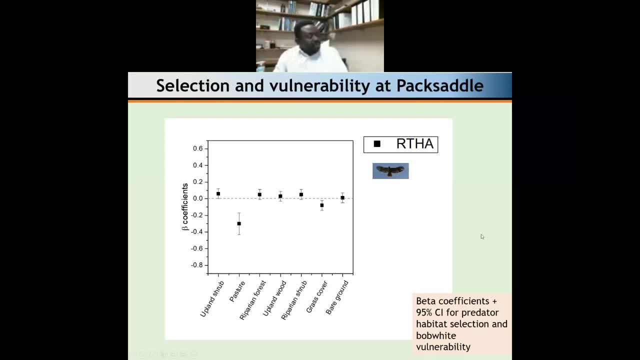 will represent the mean of selection. So if we have any of these dots above that line, So if we have any of these dots above that line, it means that that habitat is being preferred and selected for by these predators. and then, if it's beneath that line, 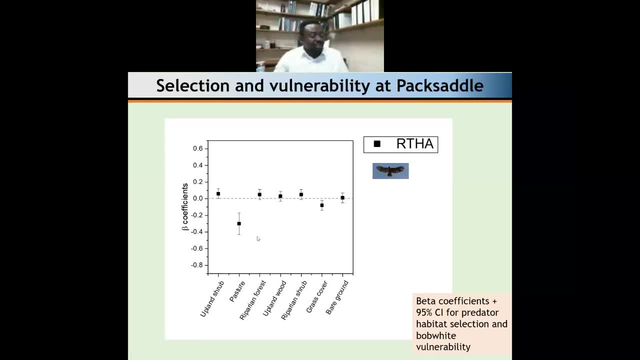 it means the habitat variable or the vegetation variable, rather, is not selected, it's just avoided. And of course, if it's within that line, then we're saying that that selection is not significant. So let's start with red-tailed hawk here. 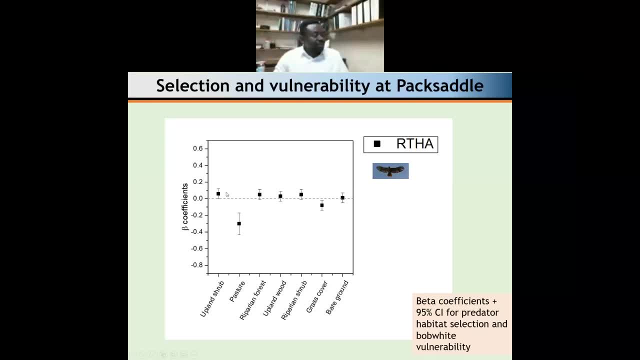 So what we see is that red-tailed hawk prefer these upland shrub areas, avoided these grass cover areas and did not show any selection for big grounds. They avoided pasture areas. It looks like they selected more of riparian forest areas. 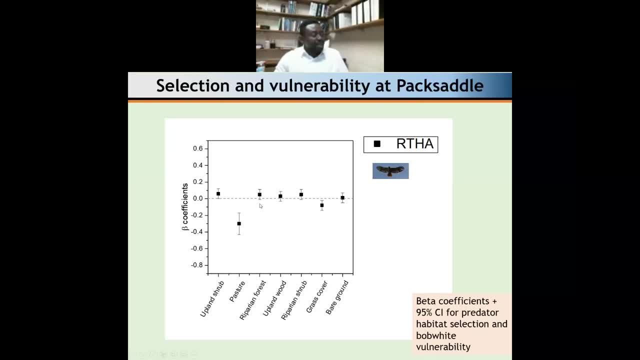 but that was not significant. And upland woody vegetation too was selected for, but not significantly different from avoidance. And all of this result represents selection at back saddle. When we put areas to that graph, that's what we see. So we see that in some areas. 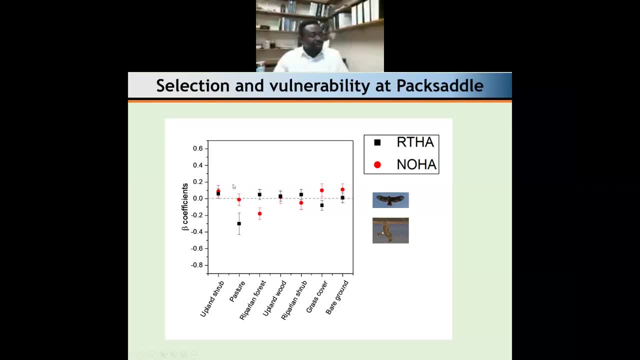 there is overlap in selection between areas and red-tailed hawks. Now let's put risky areas, as these areas who were recorded Significant mortalities of bulk white quail. You will see again where we have these points above the line means. 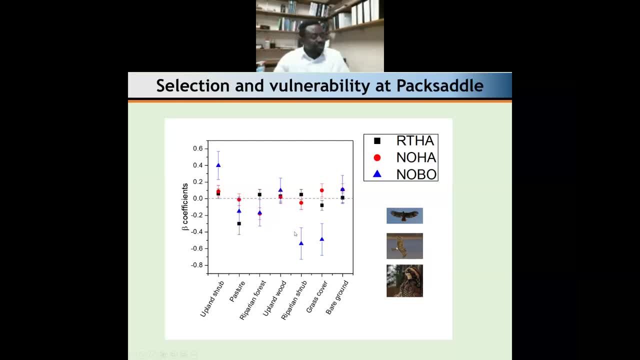 where we are dying significantly And where we have them below the line means where we're doing very well, And that's what you see. So if you were to circle those out, you will see that all the areas where we have quail dying significantly are areas 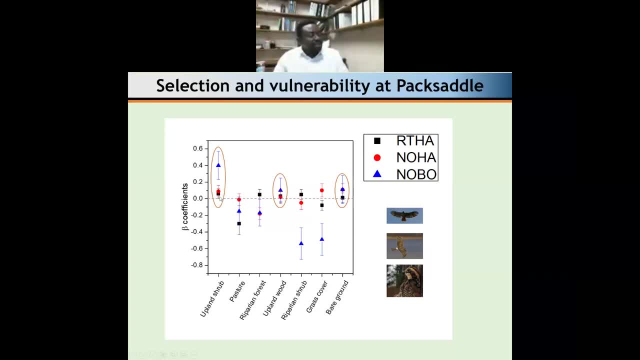 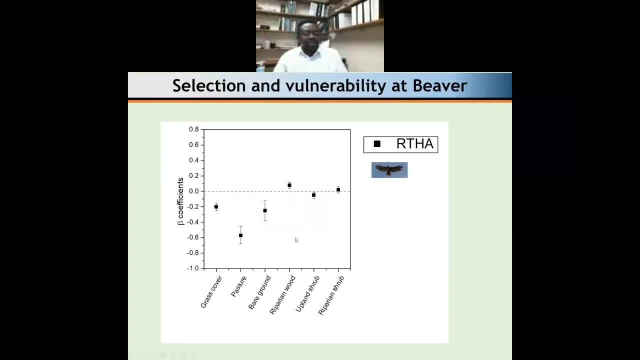 where red-tailed hawk and northern harrier appear to overlap in their selection. However, if we move to Beaver River, which is less complex or less heterogeneous, in this case we'll see different patterns And we see that areas where quail were dying well. 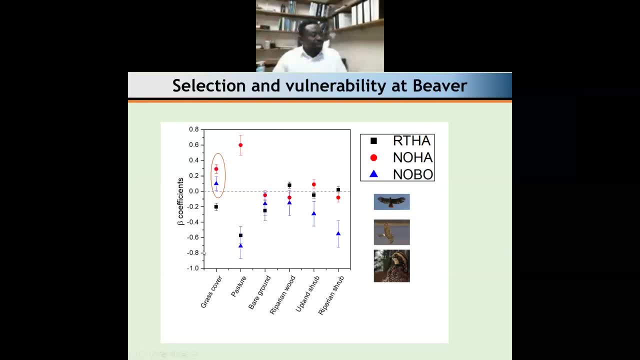 significantly low. In fact, it was just one area, which is areas with that were mostly grasslands, And in that area we could only attribute one predator to mortality, And that would be the northern harrier, And harriers don't breed in backside or down south. 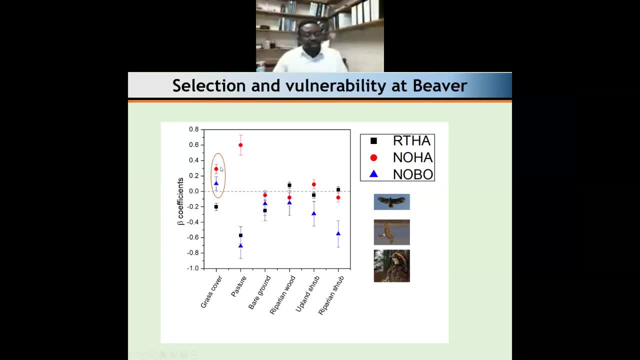 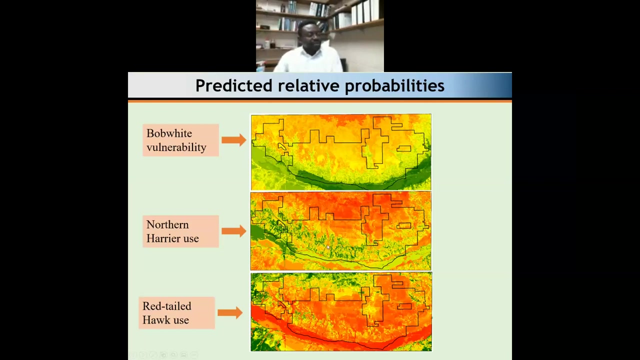 In fact they don't breed anywhere down south, So it means that this mortality rates from predation is only apparent during the non-breeding season of quail. So quail are not having a lot of pressure from predators. I don't know how much time we had. 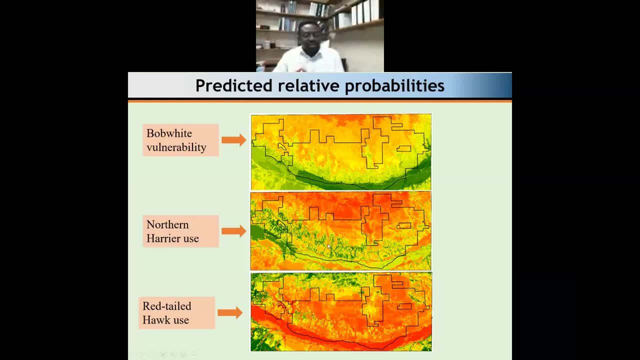 but all of this is trying to present this information in graphical way such that it can be utilized easily by wildlife managers for decision making. So if we don't have time- and I assume it's almost six o'clock here for me- I would just keep all of those complex analysis. 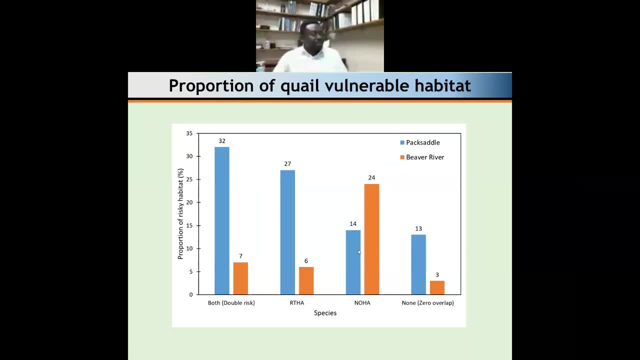 But overall, what I want us to take home is that at a place like Pack Saddle, we try to classify risky areas within the landscape, And we saw that for the entire landscape when it comes to predation. about 32% of the entire landscape is an area. 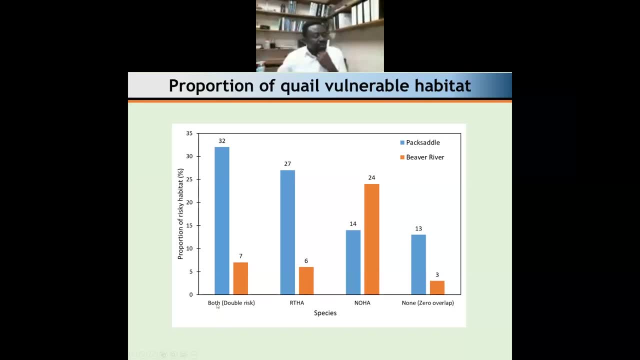 where both red-tailed hawk and northern harrier overlap greatly and might present significant risks to quail And we see that high for red-tailed hawk but not very much for harriers. Again, remember I said harriers are non-resident birds. 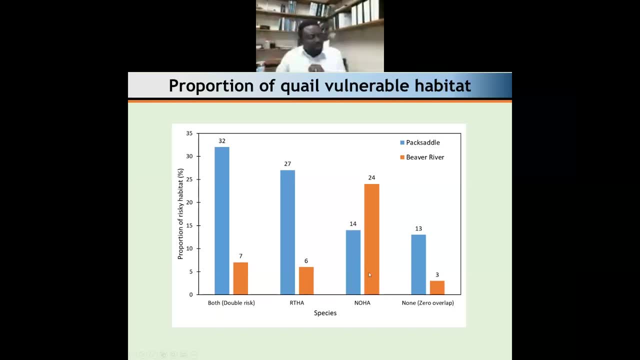 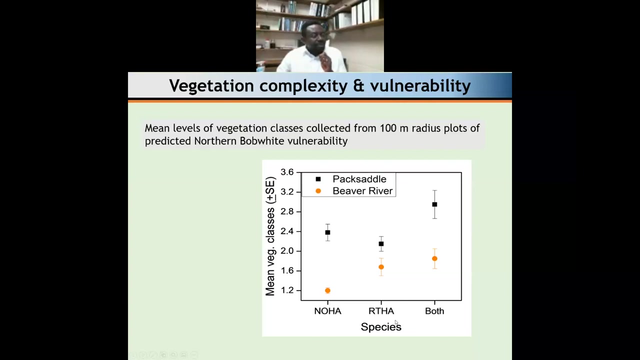 so they come in just during the winter and we have more of them at Beaver River. So at Beaver River you can say that about 25 or 24% of the area is open to harrier predation risk. In conclusion, we try to look at how complex the habitat was. 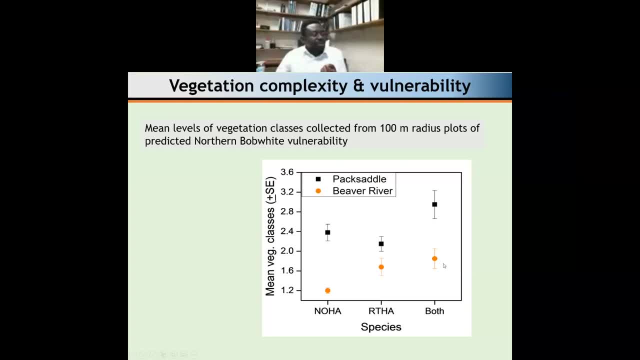 at each of the sites that quail were dying. So for each spot where we had mortality of quail we put 100 meters radius buffers around those areas to characterize how complex those vegetation was around those areas. And we end up with this. we say that at Pack Saddle. 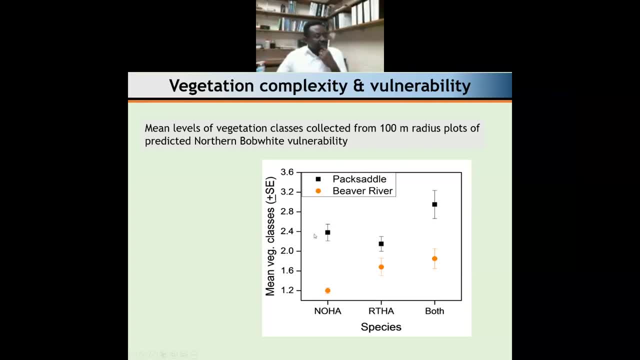 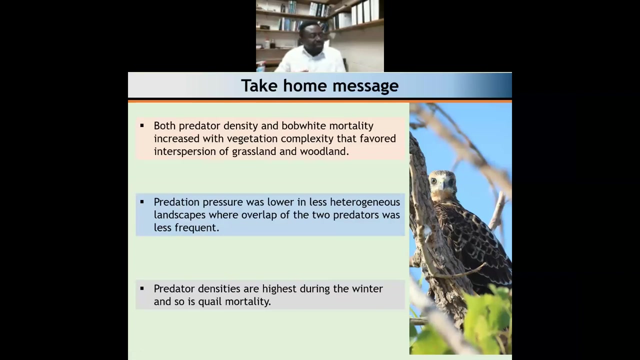 wherever quail were dying as a result of northern harrier predation or red-tailed predation. all of those areas were way more complex in terms of vegetation structure compared to Beaver River. So I will say, indeed it appears that raptor densities 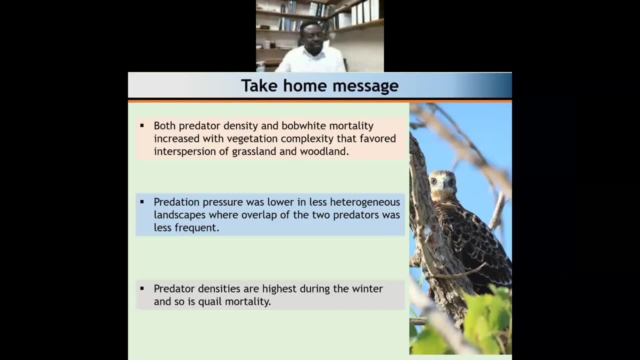 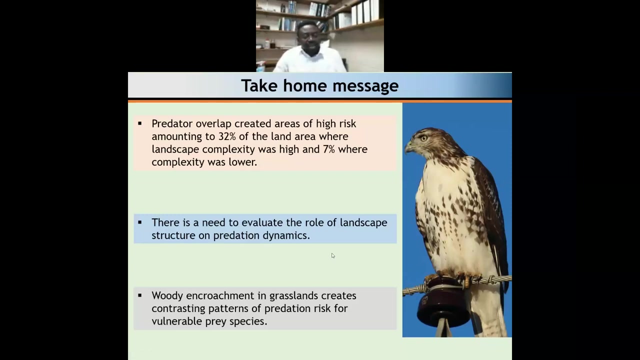 were high in these areas, especially during the winter, and those could somehow impact on quail survival. And then we're able to quantify that landscape of predation risk that managers could pick up and use to implement management outcomes or management planning that's could reduce predation rates. 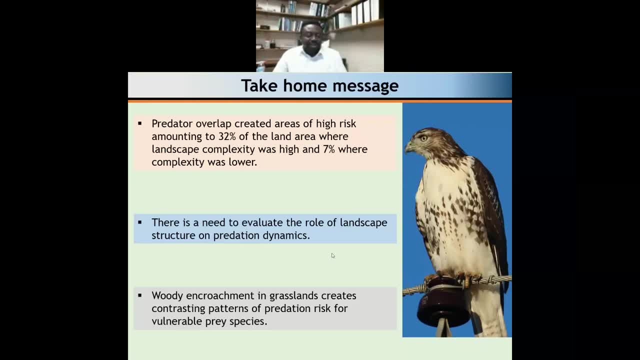 Like Dory says, people are often very happy to say, OK, maybe let's reduce raptor population because there impact it's getting on quail. But that's not what we are saying in this study. What we are saying is that change in the landscape structure. 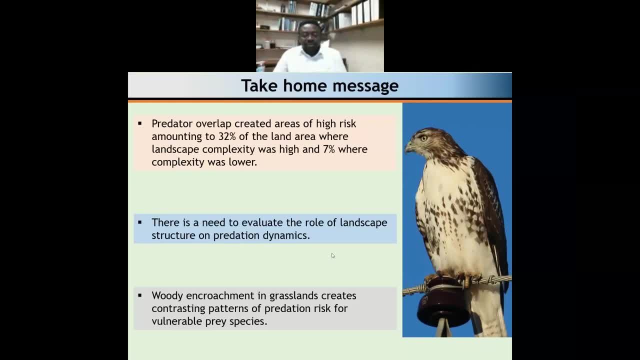 external area fuelling全部 koi. the overlying of the predator isjsie risk areas for keeping에는 imumalechiazu from traditional structures to some encroachment, like woody vegetation, can change the way species interact on the landscape. 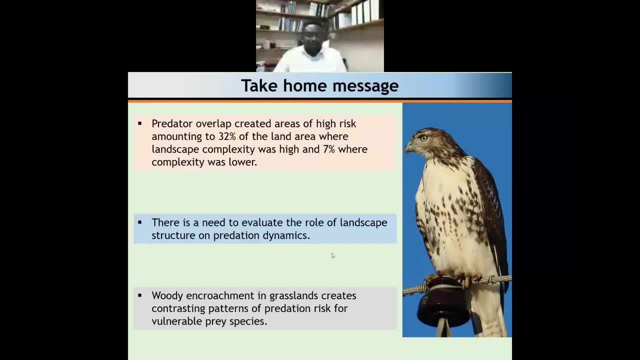 and might increase predation risk. So what we need to do is reduce that complexity by somehow removing woody encroachments from grassland ecosystems. I think that's where I'll stop, And if we have time for questions, I'll probably take some questions. 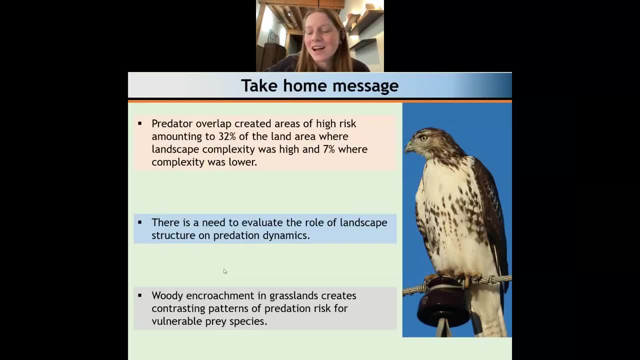 Alrighty. So thank you, Fidel, for that presentation. Yeah, so we'll take a few questions, So if you have any, please pop them in the chat. For now I have one question for Tori, asking if you've ever witnessed a lek being flushed. 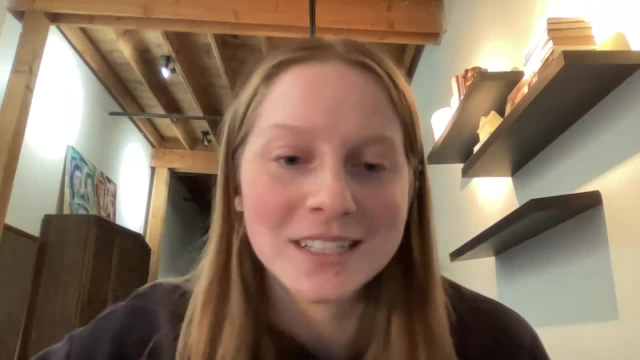 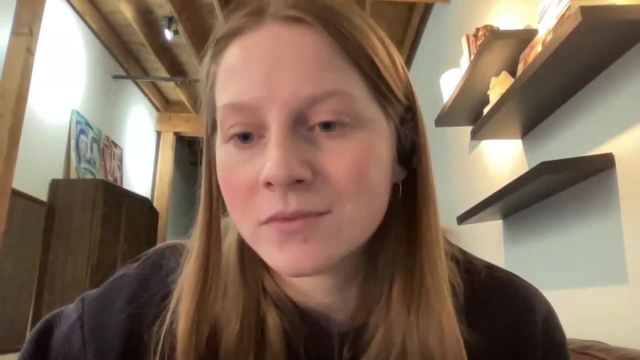 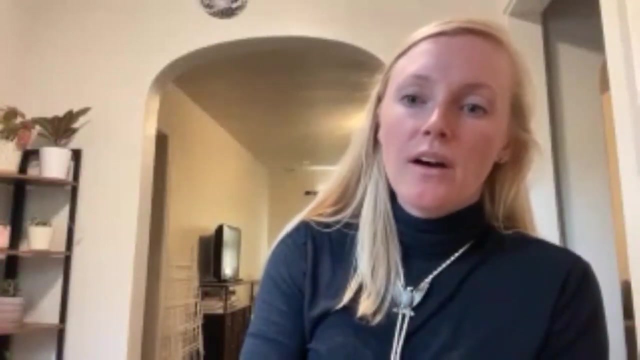 by an eagle attack. They personally have seen one on one occasion, but the golden eagle was unsuccessful, So I didn't personally witness that this spring, but my technician did witness that, where golden eagle flew low over the lek and all the grouse flushed. 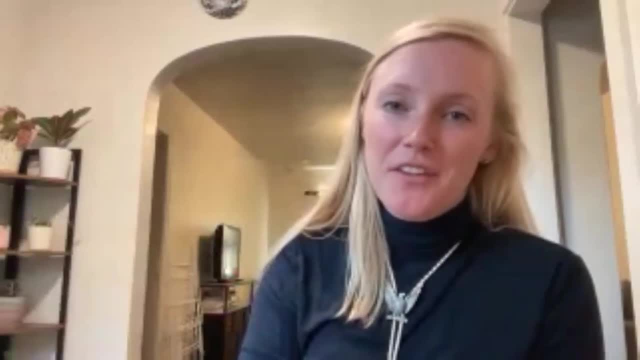 And then the golden eagle actually perched on the ground near the lek and the sage grouse never came back to the lek that day, And that's one of the things I'm interested in is, if they flush, do they ever come back? 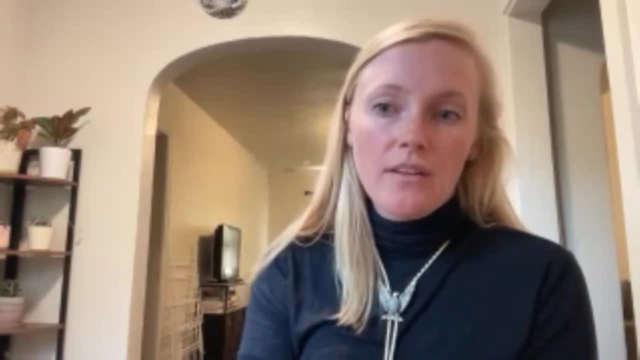 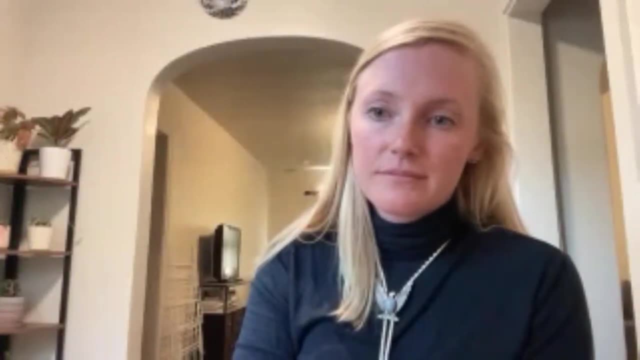 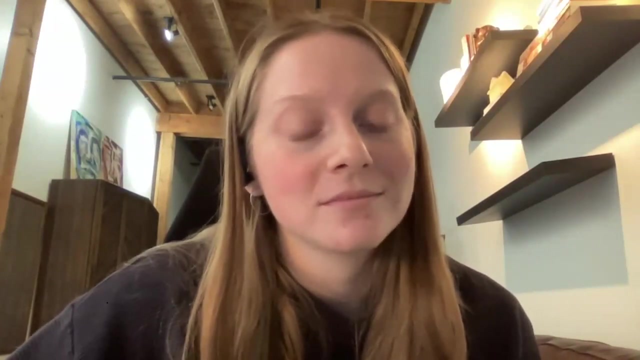 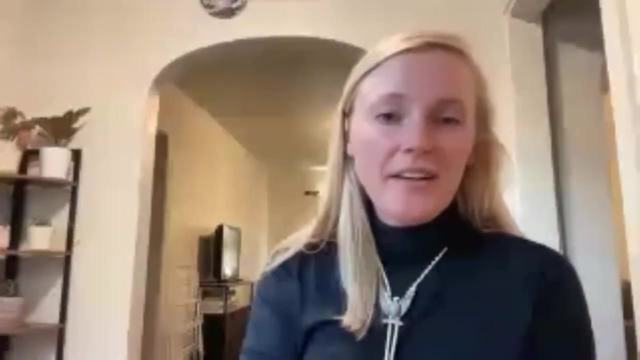 once the predator leaves, Or do they not return at all until the next morning? I have another question for Tori asking what is the ratio female versus male GSG in your area? So, based on the first season, that really depends on the day. 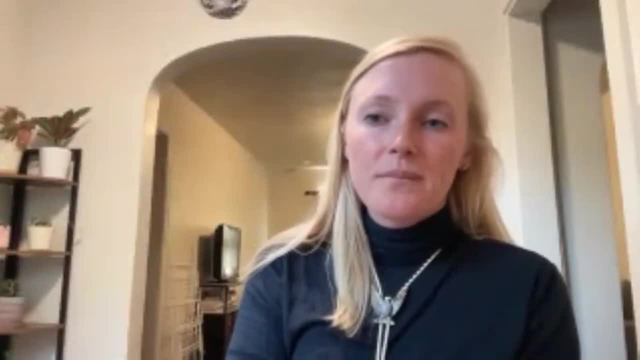 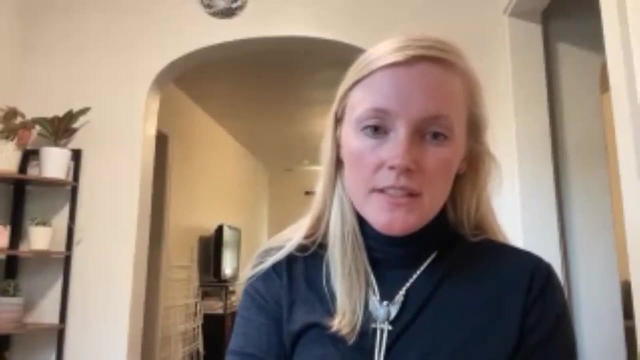 and the period of the lek season. Seven to 10 females And we had accessory male atttendants, and that just the spring. So does that��? 연 catells? similarly? No, that's just for the season. So early on we had mostly males coming. 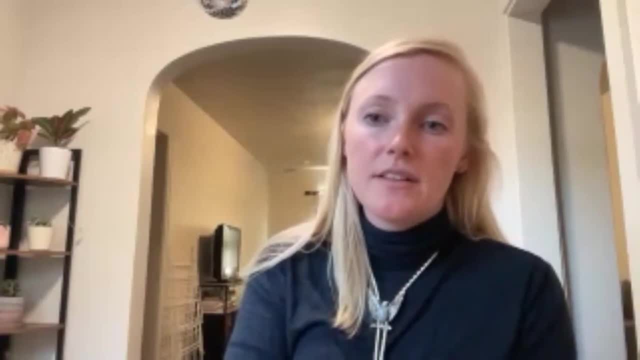 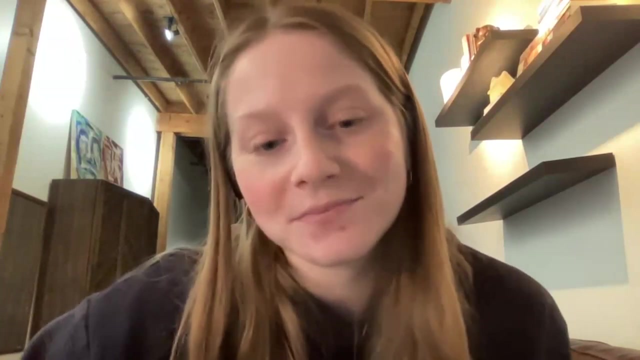 and just a few females, And then, probably around the end of March, early April, we had peak female attendants And then, once again, the females started to trail off. is the work that you're focusing on these days, since that was your PhD project? 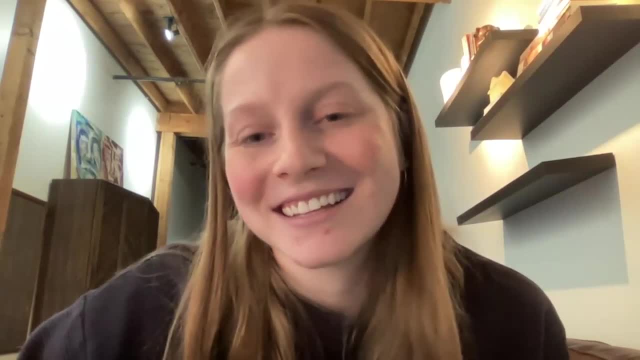 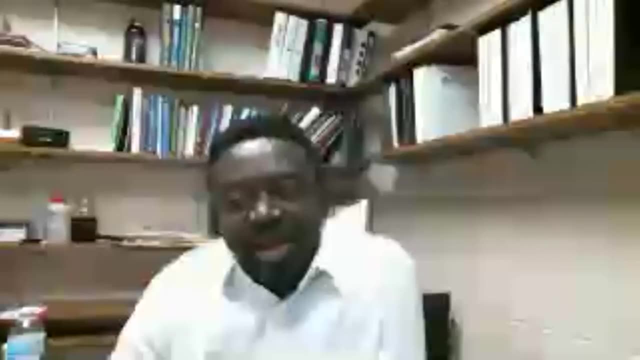 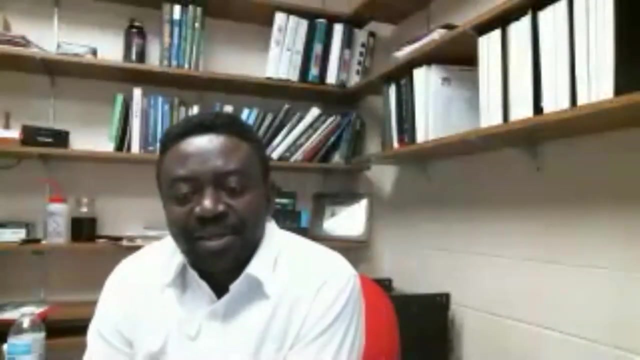 Oh, I can't hear you, Fidel, you're muted. Oh yeah, so I'm currently doing a few other projects. So I'm interested in fires in savanna ecosystems, So I'm still working with grass land or grand dwelling birds, still galley farms. 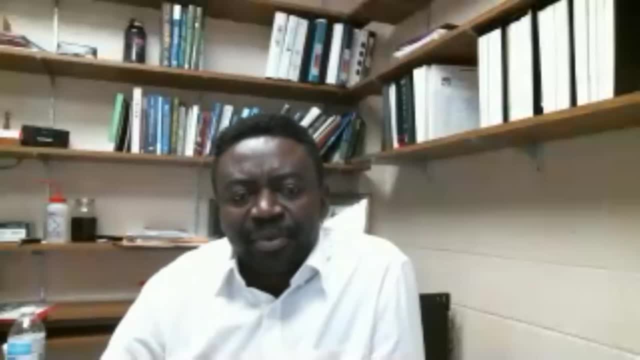 So I'm looking at how fires impact galley farm's habitat selection and protection rigs, but this time around in savanna ecosystems, So I have a graduate student working on that. I'm also interested in some social ecological stuff, So looking at how we can encourage young people. 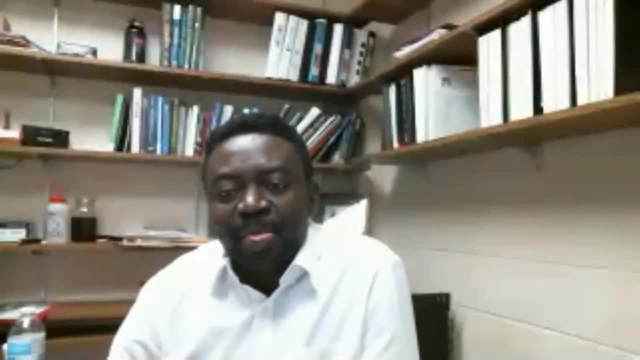 to join this conservation career. So I'm looking at things like social media video and social media Video games could impact how much time kids or youth spend outdoors, because we want youth to spend more time outside for many reasons- for the health benefits that it provides. but also because provides funding for conservation in the long term. State agencies rely on things like resources, monies that comes from game hunting and fishing to fund conservation research And, if we are not having people spending time outdoors or buying those licenses, paying those fees. 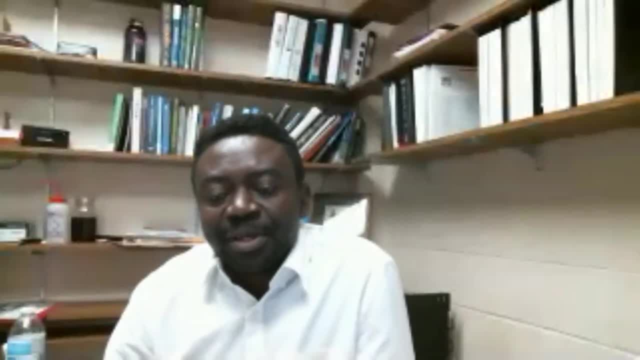 we might just run short of monies for conservation in the future, But that's something else I'm interested in. I'm also still interested in how oil and gas structures are impacting on habitat availability for birds in savanna, And I'm interested in how we can help. 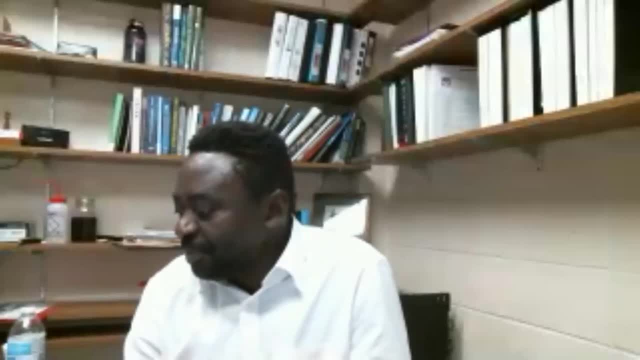 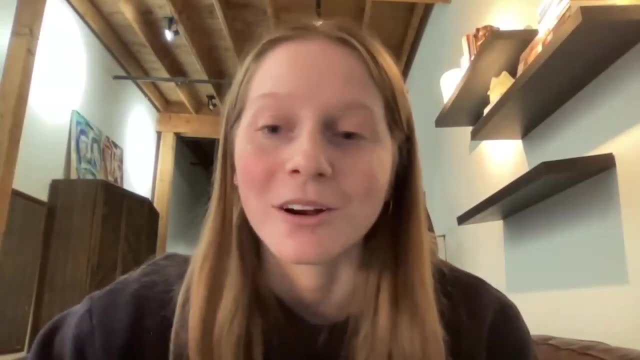 to help other species, like animals and animals that are still in western Oklahoma. Great Well, I want to be mindful of everyone's time, So I'm going to thank everybody for joining us today. Once again. a recording of this lecture will be posted. 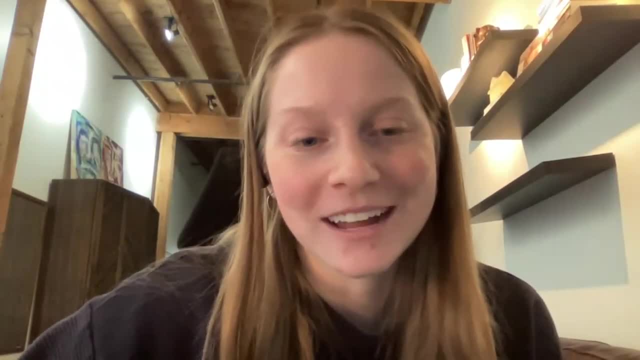 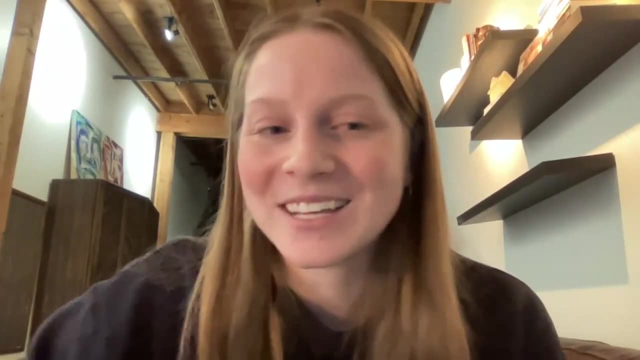 on our YouTube channel And thank you again to Fidel and Tori for putting on such a great talk for everybody today. Thank you, Thank you everybody. Have a good one, Thanks.